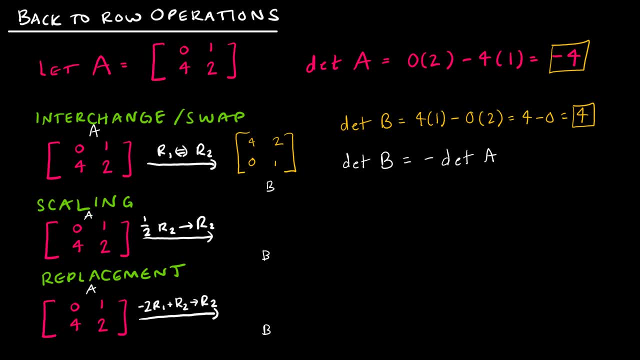 So whatever you had for A, you can change the sign and that's going to be the new value, or the value of the determinant for your new matrix. So there's one rule. Let's take a look at the next one. This is scaling. 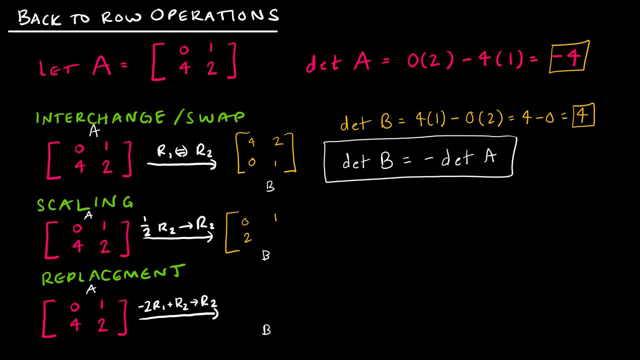 So if I take one half of row two, that gives me two and one. The determinant of B is zero, 0 times 1, minus 2 times 1, which is 0 minus 2, or negative 2.. So it looks like what happened is: I took 1 half times row 2,. 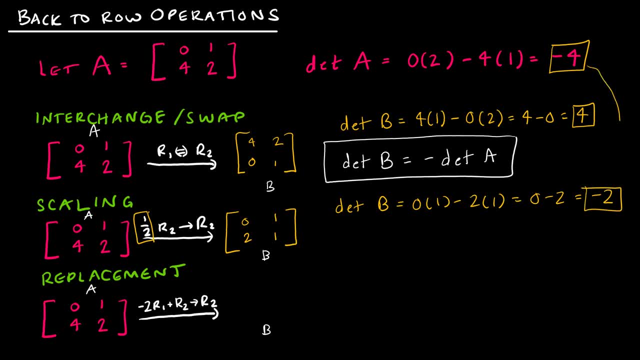 and what happened to get negative 2?? From 4 to negative 2, it looks like I took 1 half of negative 4 to get negative 2, and that is in fact the rule. So the determinant of B, your new matrix, is going to be equal to C times the determinant of A. 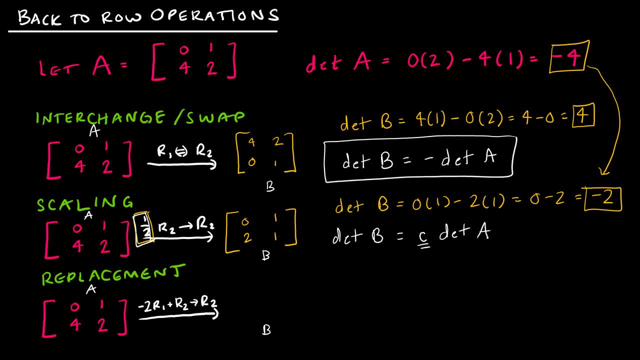 and C, of course, would be whatever value you have here that you are multiplying by your scalar in your row operation: Great, so just one more to go. Let's take a look: This is replacement, and so we're going to take in this case. 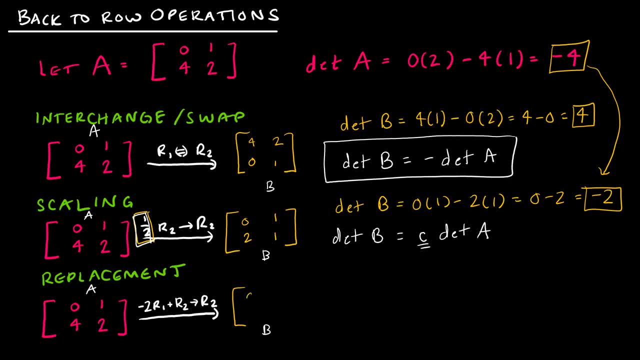 say negative 2, row 1.. So row 1 remains the same, Row 2 would be 0 plus 4,, which is 4, and negative 2 plus 2, which is 0.. So let's find the determinant now of my new matrix B. 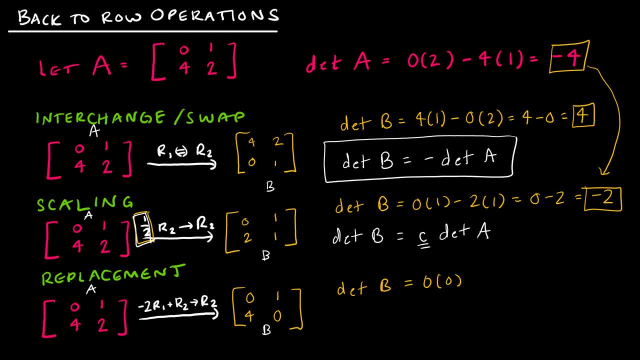 My determinant of B would be 0 times 0, minus 4 times 1,, which is 0 minus 4, or negative 4.. And it looks like not a darn thing happened, and that is in fact the case. 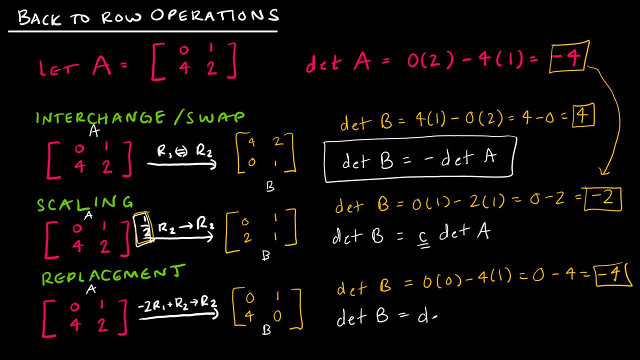 So the determinant of B would be 0 times 0, minus 4 times 1,, which is 0 minus 4, or negative 4.. So the determinant of B is going to be equal to the determinant of A, So a replacement is not going to change anything for your determinant. 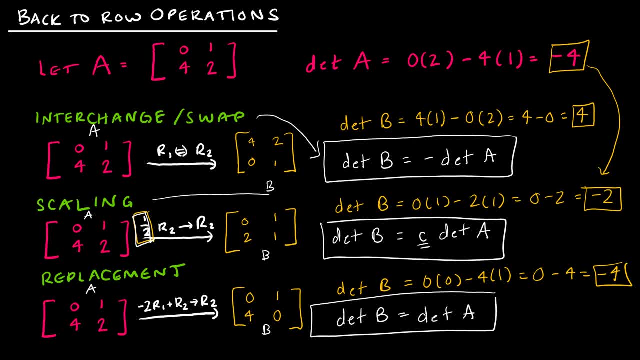 So here's our rules. Make sure you keep straight which one belongs to which. Now you might be asking: why do I care? Can't I just find the new matrix and find the determinant of that matrix? Well, sure, If you've got a 2 by 2 matrix, absolutely. 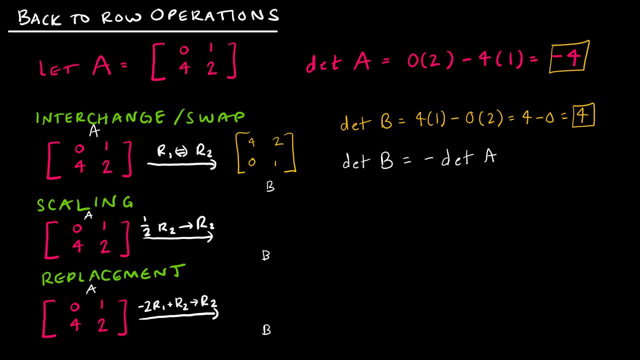 for A, you can change the sign and that's going to be the new value, or the value of the determinant, for your new matrix. So there's one rule. Let's take a look at the. the next one: This is scaling. So if I take 1, half of row 2, that gives me 2 and 1.. The determinant: 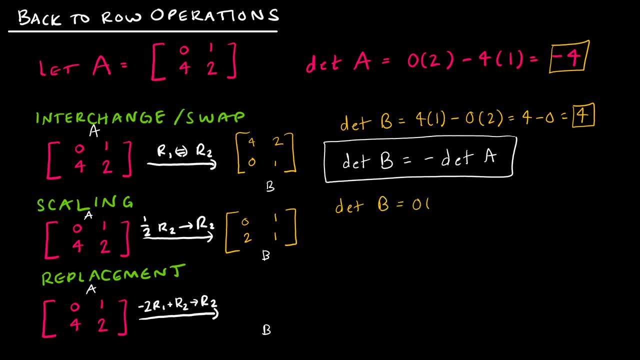 of B is 0 times 1 minus 2 times 1,, which is 0 minus 2 or negative 2.. So it looks like what happened is I took 1 half times row 2, and what happened to get negative 2? From 4 to negative 2,. 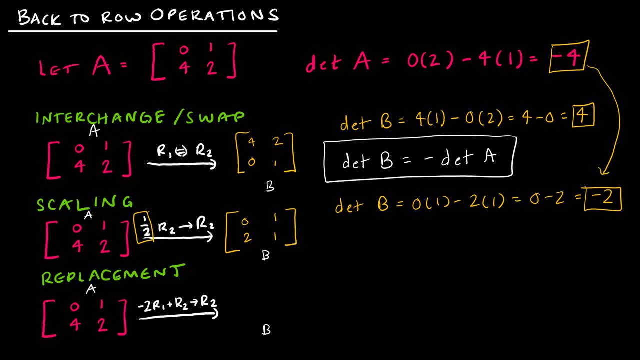 it looks like I took 1 half of negative 4 to get negative 2, and that is in fact the rule. So the determinant of B, your new matrix, is going to be equal to C times the determinant of A, and C, of course, would be whatever value. 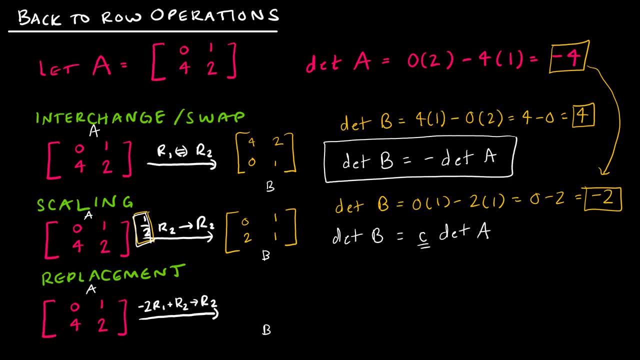 you have here that you are multiplying by your scalar in your row operation. Great, So just one more to go. Let's take a look: This is replacement, And so we're going to take, in this case, say, negative, 2 row 1 plus row 2.. So row 1 remains. 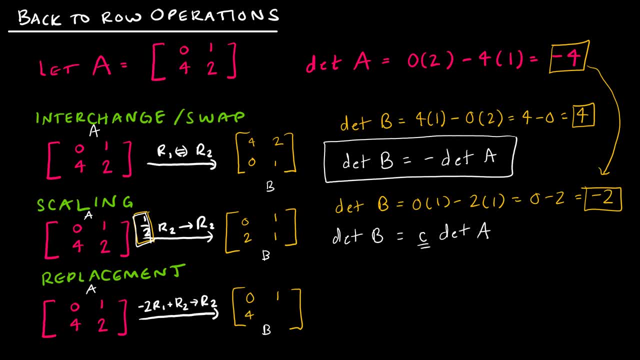 the same Row, 2 would be 0 plus 4,, which is 4, and negative 2 plus 2,, which is 0.. So let's find the determinant now of my new matrix B. my determinant of B would be 0 times 0 minus 4 times 1,, which is 0 minus 4 or negative. 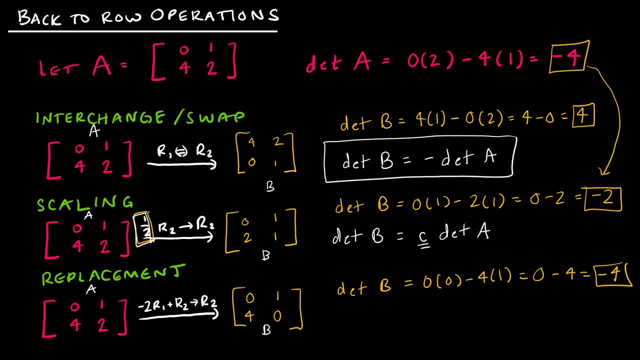 4. And it looks like not a darn thing happened, and that is in fact the case. So the determinant of B is going to be equal to the determinant of A, So a replacement is not going to change anything for your determinant. So here's our rules. Make sure you keep straight which one. 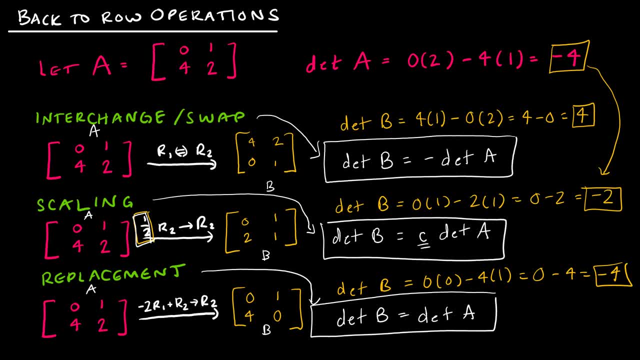 belongs to which. Now you might be asking: why do I care? Can't I just find the new matrix and find the determinant of that matrix? Well sure, If you've got a two by two matrix, absolutely No point in dealing with these pesky little properties. But that's not going to be the case. 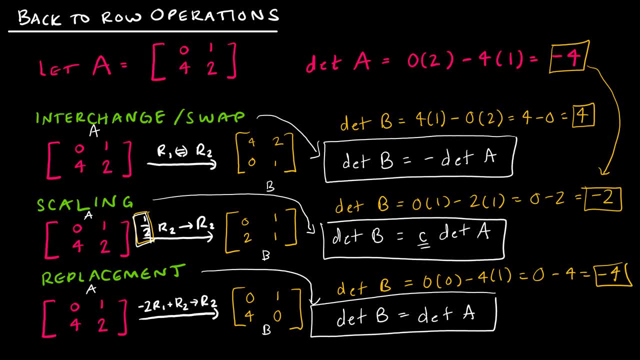 No point. No point in dealing with these pesky little properties. But that's not going to be the case, because we're going to give you, say, a 4 by 4, or a 5 by 5, or a 6 by 6.. 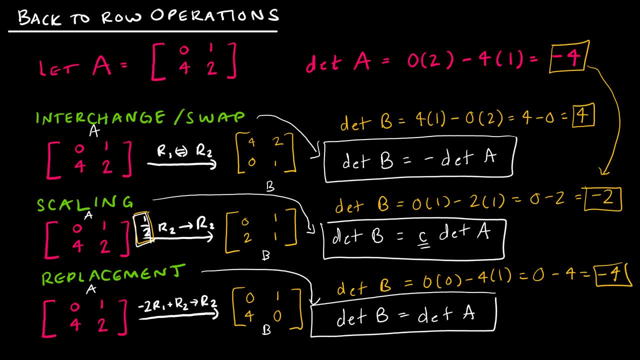 And our goal is to be able to take something that's very complicated like that and to just find out what is going to happen to the determinant, so that I can sort of it's sort of like a puzzle where I'm finding all of the steps and sort of undoing those steps. 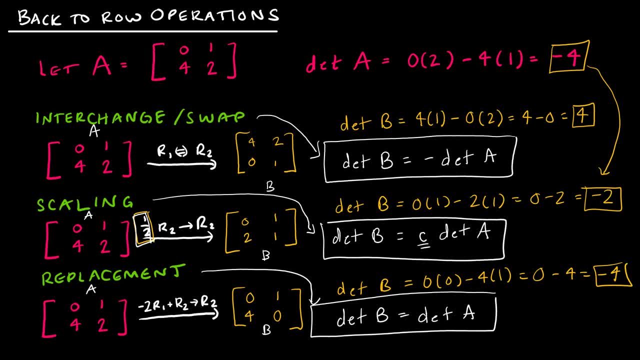 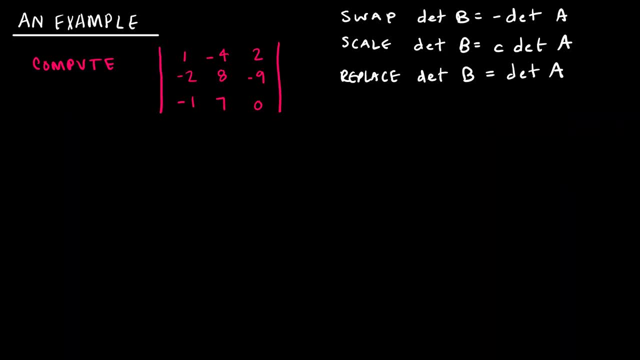 so we'll make much more sense when we do an example together. So let's just get to that. Here's an example for us to go through together, and this is a fairly easy example to begin with, but I just want to get you used to the idea. 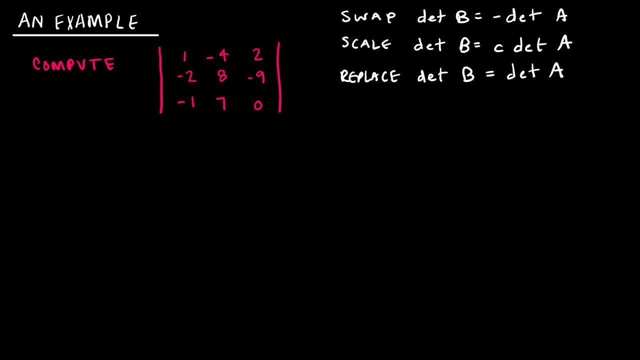 So what I'm trying to do is I'm trying to compute the determinant and I'm just going to call it matrix A. So if I want to find the determinant of A, it's telling me to, of course, find the determinant of this matrix. 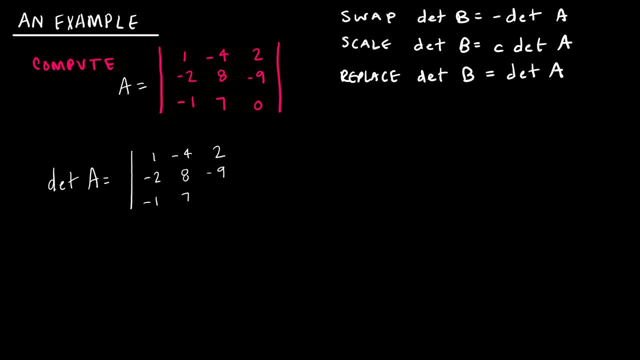 Now, could I find the determinant of this matrix using cofactor expansion? Of course I could, but I don't want to do that. I want to use these properties of the determinant to simplify. Let's do some row operations. So I'm going to basically do a couple of row operations here, just like you normally. 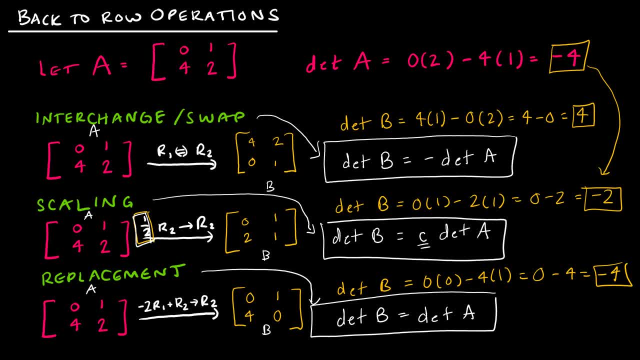 because we're going to be dealing with a two by two matrix. So we're going to be dealing with a two by two matrix. So we're going to be dealing with a two by two matrix, So we're going to be giving you, say, a four by four or a five by five or a six by six, And our goal is to be able. 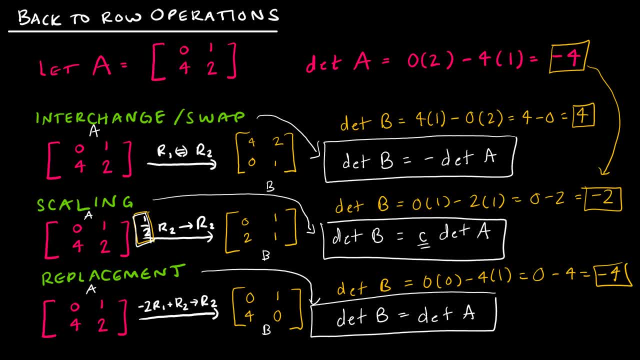 to take something that's very complicated like that and to just find out what is going to happen to the determinant, so that I can sort of it's sort of like a puzzle where I'm finding all of the steps and sort of undoing those steps. So it'll make much more sense when we do an example. 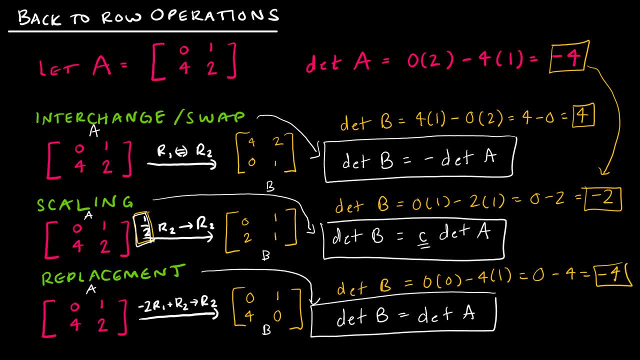 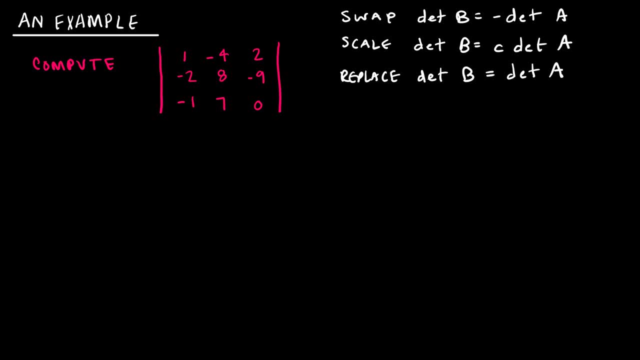 together. So let's just get to that. Here's an example for us to go through together, And this is a fairly easy example to begin with, but I just want to get you used to the idea. So what I'm trying to do is I'm trying to compute. 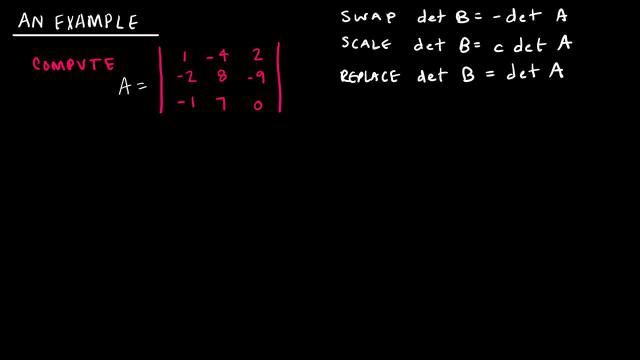 the determinant, and I'm just going to call it matrix A. So if I want to find the determinant of A, it's telling me to of course find the determinant of this matrix. Now, could I find the determinant of this matrix using cofactor expansion? Of course I could, But 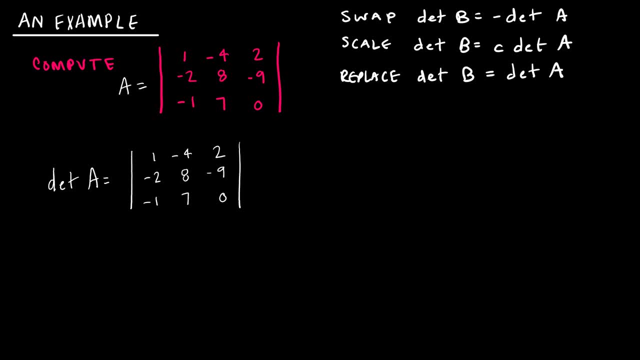 I don't want to do that. I want to use these properties of the determinant to simplify. Let's do some row operations. So I'm going to basically do a couple of row operations here, just like you normally would. So this is stuff you're totally used to at this point. 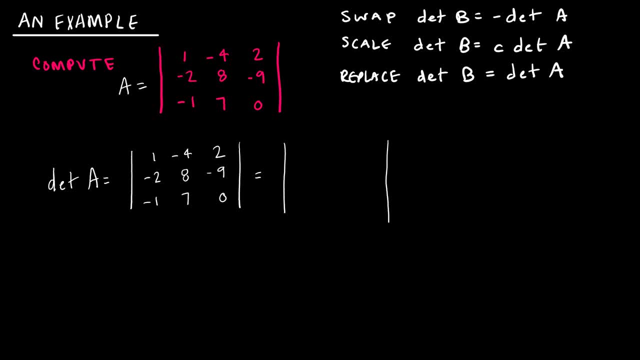 I'm trying to get this to be a row, So I'm going to do a couple of row operations here, not into reduced row echelon form, but just into triangular form. And again, that will become clear once we get to the end of this question. 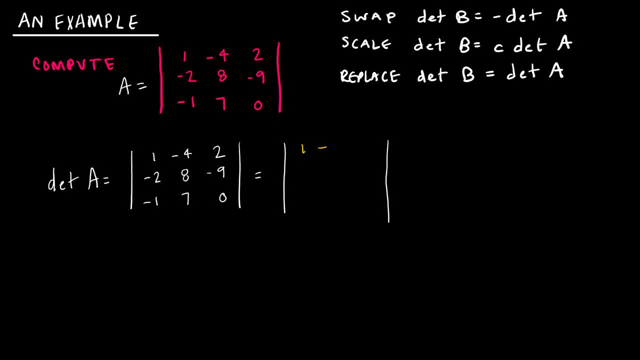 So I'm going to leave my first row the same. My second row. that's a weird one, So let's redo that one. My second row: again. I'm trying to get a zero here and a zero here. So my second row. 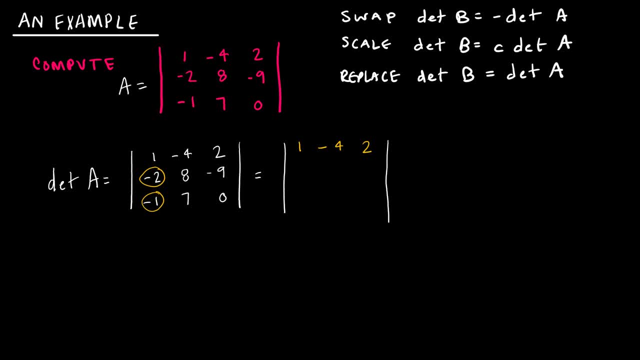 I'm going to take two times row one plus row two to be my new row two. So two times one is two plus negative two. Two times negative four is negative eight plus eight. Two times two is four plus negative nine. And then I'm going to take row one plus row three to be my new row three. So one and negative one. 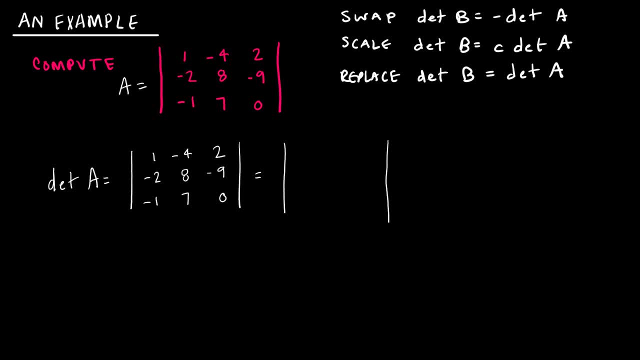 would. So this is stuff you're totally used to. at this point I'm trying to get this not into reduced row echelon form but just into triangular form, And again, that will become clear once we get to the end of this question. 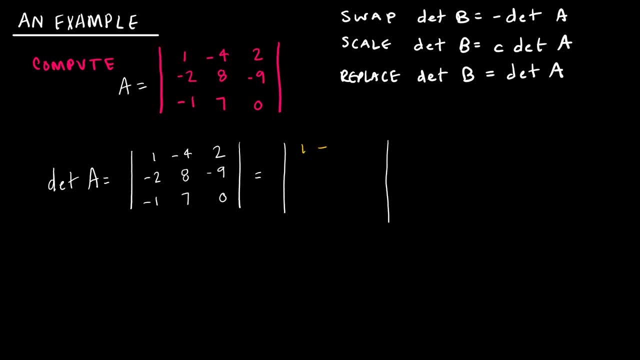 So I'm going to leave my first row the same. My second row: that's a weird one, so let's redo that one. My second row: again, I'm trying to get a 0 here and a 0 here, So my second row I'm going to take 2 times row 1 plus row 2 to be my new row 2.. 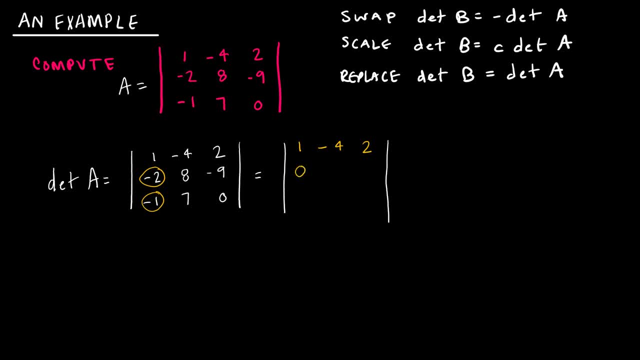 So 2 times 1 is 2 plus negative 2.. 2 times negative 4 is negative 8 plus 8.. 2 times 2 is 4 plus negative 9.. And then I'm going to take row 1 plus row 3 to be my new row 3.. 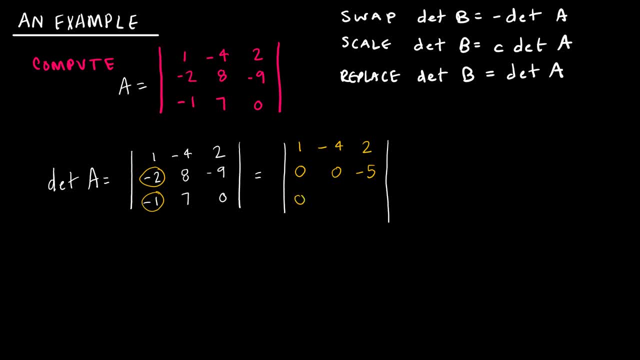 So 1 and negative, 1 is 0, negative 4 and 7 is 3,, 2 and 0 is 2.. So, before I continue any row operations, what did I just do? Which of these row operations did I perform? 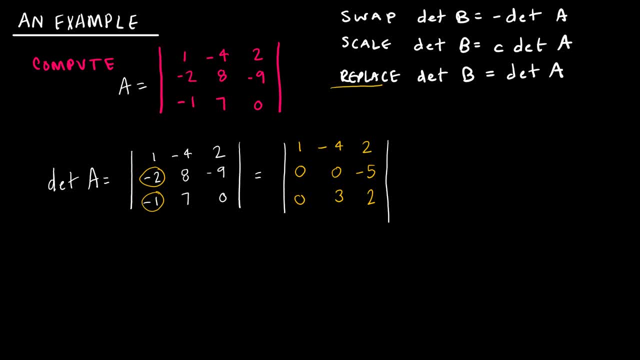 Well, to get my new row 2, I did a replacement, A replacement being that I multiplied some row by something and added it to something else, So I replaced the entire row, and I also did that for row 3.. The reason this is important is because that's not going to change my determinant at all. 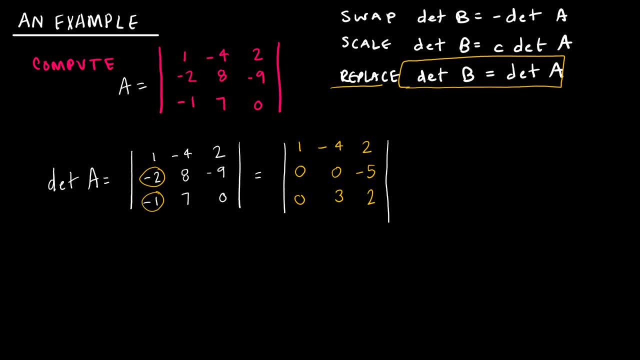 So I'm good. What am I going to do next? Because it's still not in the form I want. Right, Remember, I really want triangular form. So I'm going to keep my first row And my second row and my third row. I'm just going to swap them. 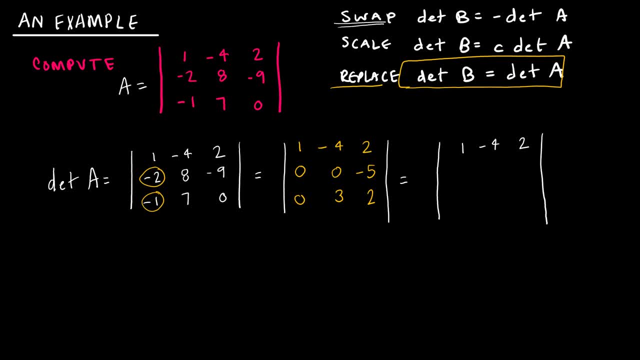 I'm going to do an interchange. Now notice I said swap. The real name is interchange, but I didn't want to write it out. I was trying to make small words. So this is 0, 3, 2, 0, 0, negative 5.. 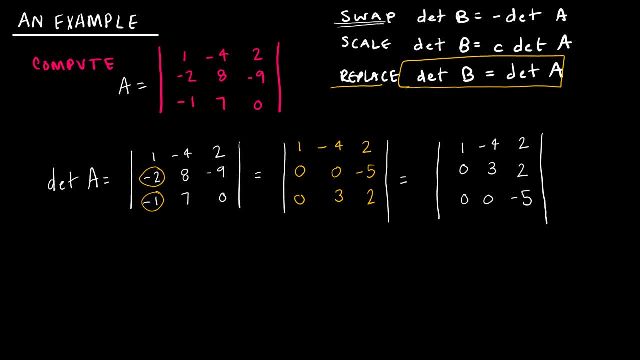 So what I've done now is I have done an interchange or swap, And the reason that's important is because it tells me that the determinant of B is going to be negative- the determinant of A, And so I have to undo that negative by putting a negative on the outside. 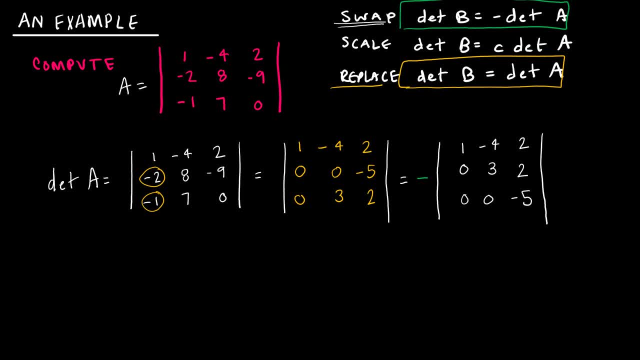 So really, this is all about undoing that so that I can get back to the determinant of A, my original matrix. Now can I find the determinant? Can I find the determinant of A at this point? Yes, I can, And here's how. 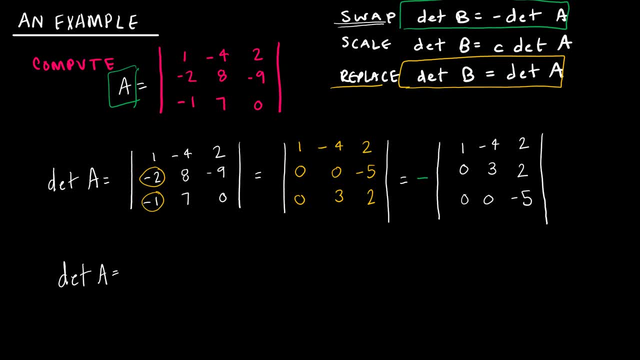 I'm going to write determinant of A. I'm just going to rewrite what I ended up with, just because I don't have enough room after that to show my work. So again, I'm leaving this negative out front, because this told me that I have to change the sign in order for it to work. 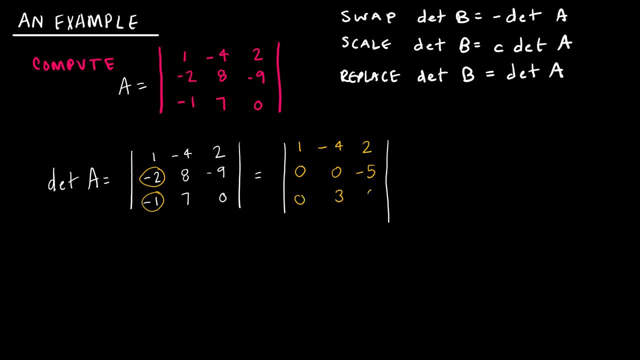 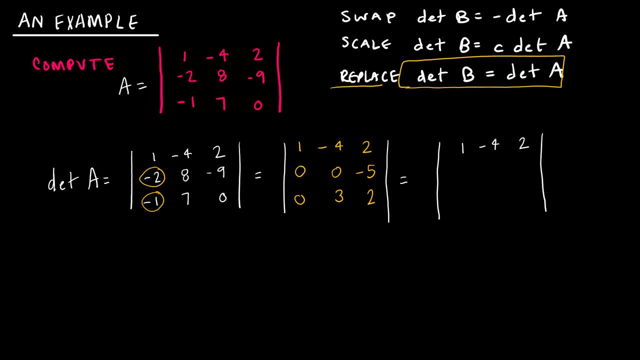 keep my first row and my second row and my third row. I'm just going to swap them. I'm going to do an interchange. Now, notice: I said swap. The real name is interchange, but I didn't want to write it out. I was trying to make small words. 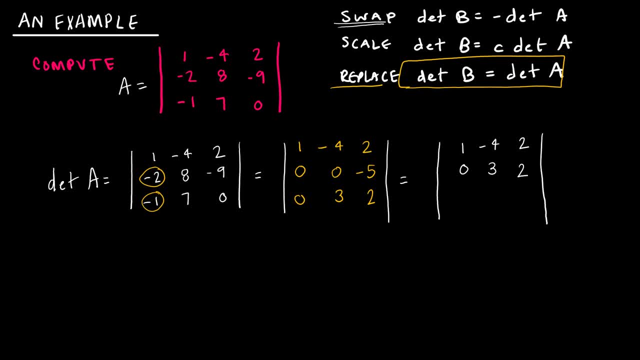 So this is 0, 3, 2, 0, 0, negative 5.. So what I've done now is I have done an interchange or swap, and the reason that's important is because it tells me that the determinant of B is going to be negative, the determinant of A, and so I 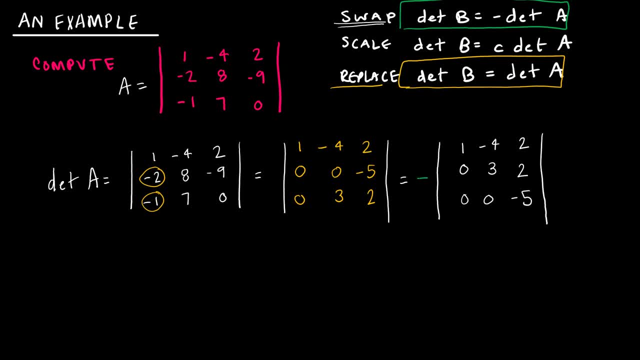 have to undo that negative by putting a negative on the outside. So really, this is all about undoing that so that I can get back to the determinant of A, my original matrix. Now can I find the determinant of A at this point? Yes, I can, and here's how I'm going to write: determinant of A. I'm just going to. 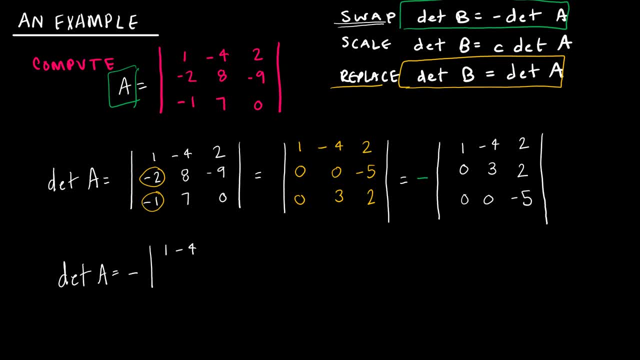 rewrite what I ended up with, just because I don't have enough room after that to show my work. So again, I'm leaving this negative out front, because it's this told me that I have to change the sign in order for it to work. and now 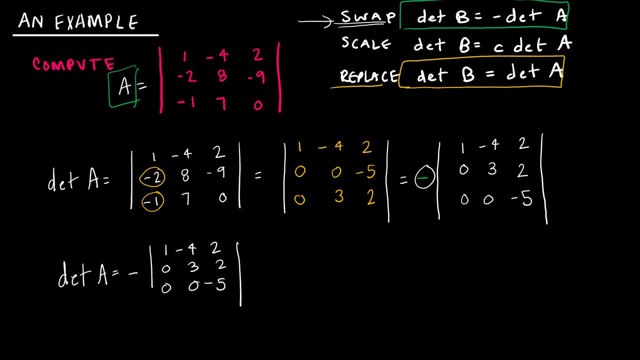 And now I'm going to find the determinant and, if you'll recall, because this matrix, which is not matrix A, it is a reduction of matrix A because I have reduced it to triangular form- I have a theorem that I ended my last video with that said: 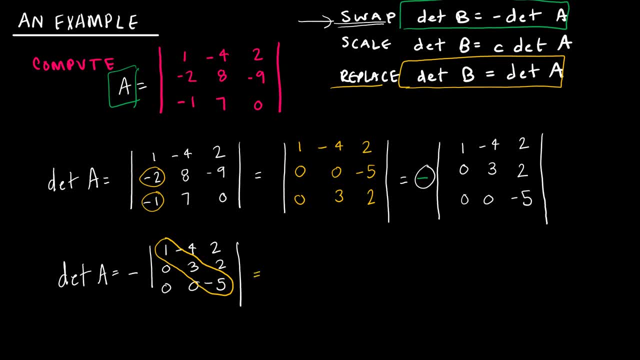 if you can get it down to triangular form, then the determinant is the product of the diagonal. So I'm going to take my negative and then I'm going to take the determinant and I'm going to take 1 times, 3 times negative, 5,. 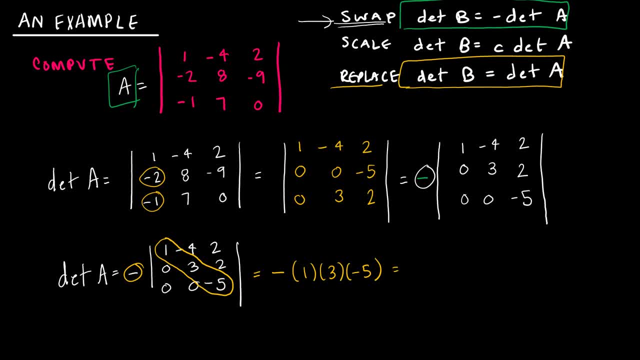 which gives me negative 1 times. 3 is negative 3 times negative, 5 is positive 15.. So could I go back to A and do it the long way and show that it is in fact 15?? Yes, Am I going to do that? 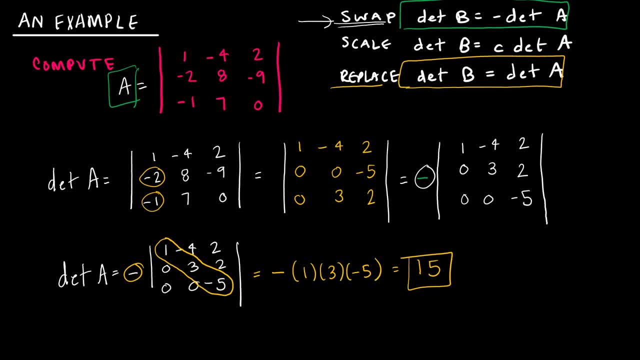 No, I will leave that for you to do, But this is how you would use these row operations or properties of the determinant To help you along the way. Now notice I haven't used scale yet. I'm saving that for our next example. 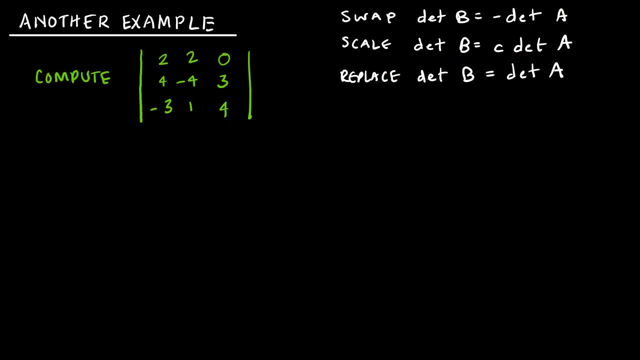 So let's take a look. Let's take a look at another example together, And again, this time I wanted to make sure we got to see what happened with scale, because this one is probably the most confusing one. So, again, the first thing I would do is I'm trying to find the determinant of A 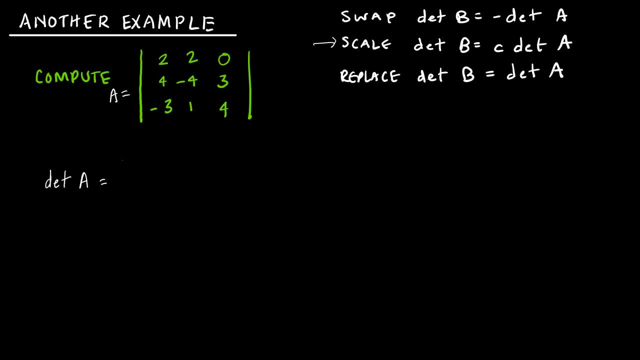 And again we're just going to call it A, And that would be to find the determinant of A, And that would be to find the determinant of A, And that would be to find the determinant of this matrix, which is our original matrix A. 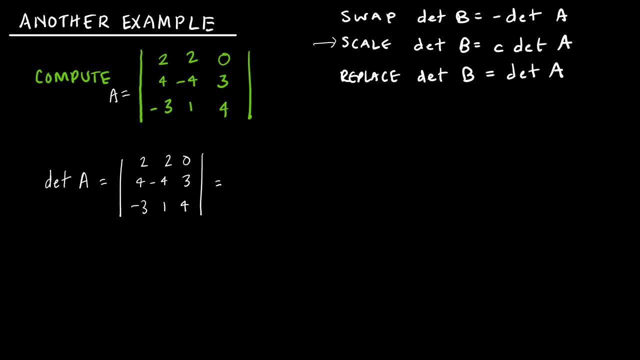 And then I'm just going to do some row operations. So again, notice, I'm not rewriting determinant each time because I'm using the square brackets. So what would I do first? Well, we obviously know we want this first term to be a one. 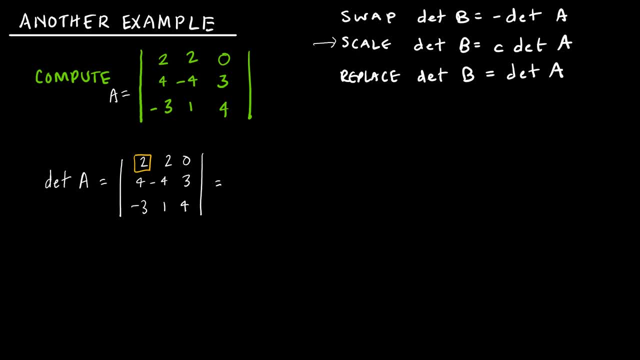 So I'm going to take one half. So if I were to write the row operation, it would be one half. Row one would be my determinant. So I'm going to take my new row, one which is a scale. Now, what does it tell me? 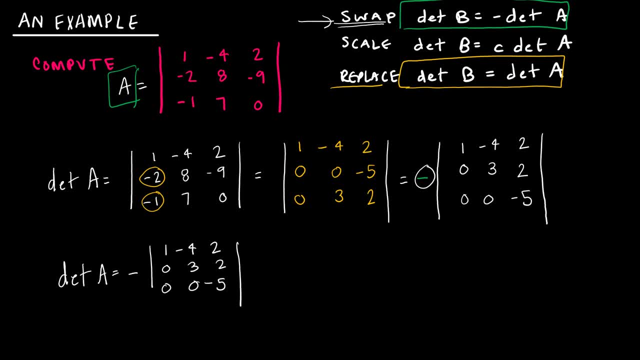 I'm going to find the determinants and, if you'll recall, because this matrix, which is not matrix A, it is a reduction of matrix A because I have reduced it to triangular form- I have a theorem that I ended my last video with. that said, if you can, 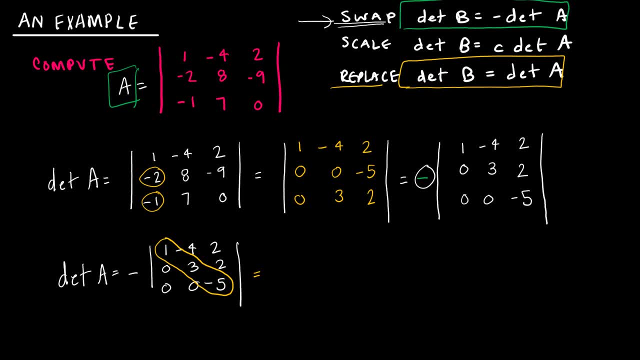 get it down to triangular form, then the determinant is the. it is the product of the diagonal. So I'm going to take my negative and then I'm going to take 1, 3, 3. times 3, times negative, 5, which gives me negative. 1 times 3 is negative. 3 times negative, 5 is. 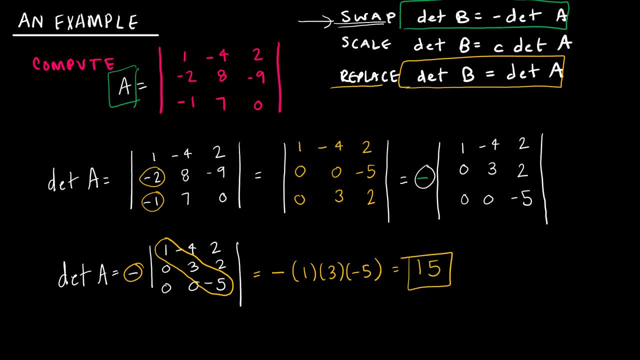 positive 15.. So could I go back to A and do it the long way and show that it is in fact 15?? Yes, Am I going to do that? No, I will leave that for you to do, But this is how you would use these. 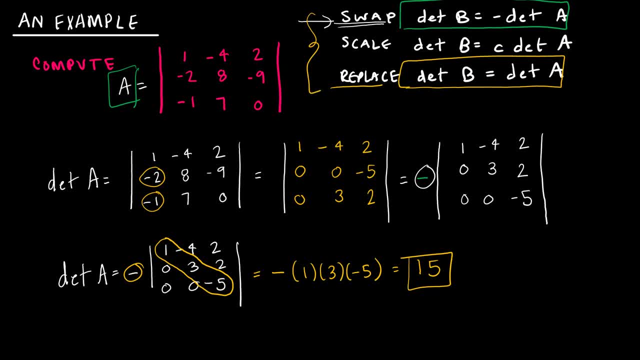 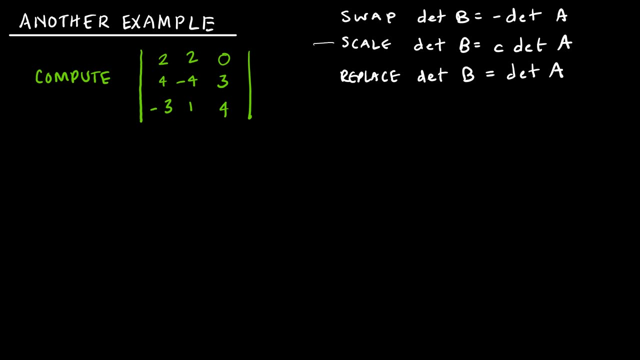 row operations or properties of the determinant to help you along the way. Now notice, I haven't used scale yet. I'm saving that for our next example, So let's take a look. Let's take a look at another example together, And again this time I wanted to make sure we got to see what happened. 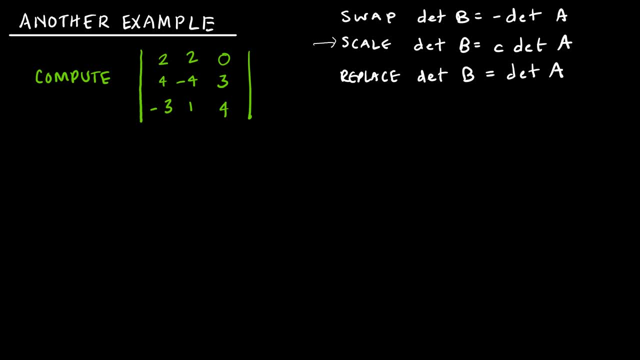 with scale, because this one is probably the most confusing one. So, again, the first thing I would do is I'm trying to find the determinant of A- And again we're just going to call it A- And that would be to find the determinant of this matrix which is our. 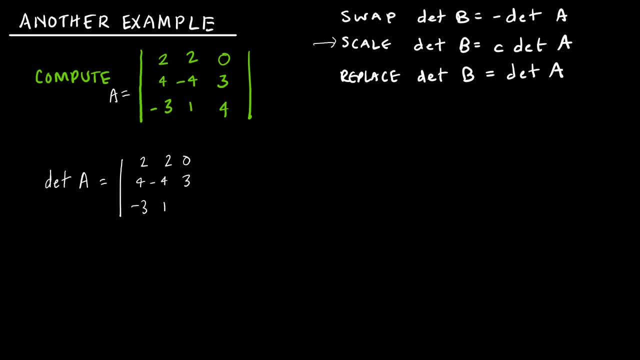 original matrix A, And then I'm just going to do some row operations. So again, notice, I'm not rewriting determinant each time because I'm using the square brackets. So what would I do first? Well, we obviously know we want this first term to be a 1.. So I'm going to take 1 half. So if I were to write 1 half, I'm going to write 1 half. So I'm going to write 1 half. So I'm going to write 1 half. So if I were to write 1 half, I'm going to write 1 half. So if I were to write 1 half, 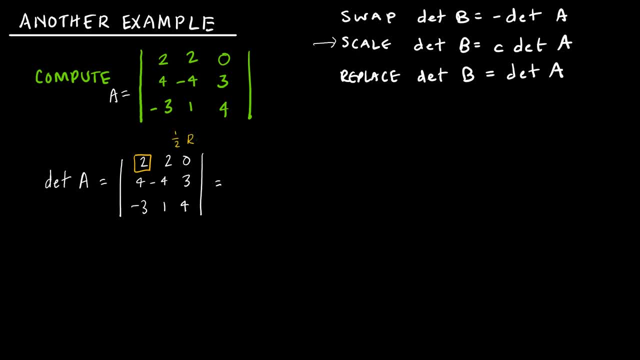 I'm going to write 1 half. So if I were to write 1 half, I'm going to write 1 half. So if I were to write the row operation, it would be 1 half. row 1 would be my new row 1, which is a scale. 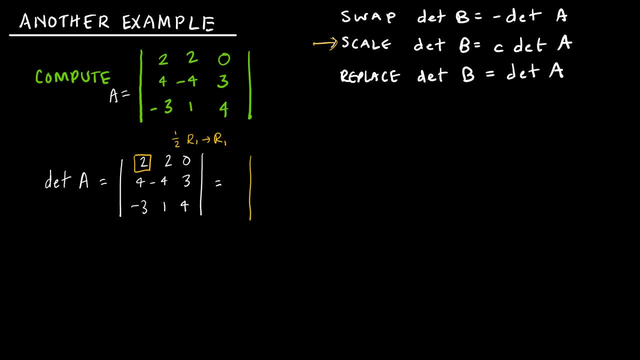 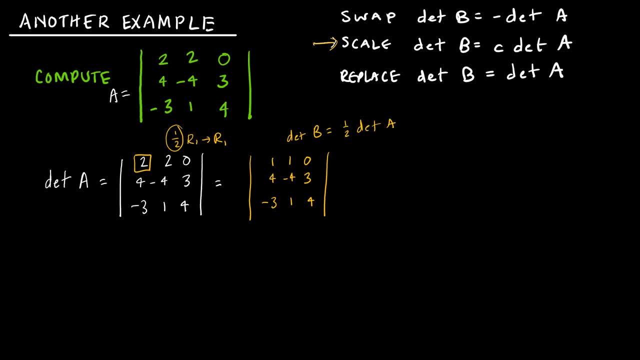 A. Here's the problem. That means a lot of people think, alright, so stick the one half here out front. but that's not the case. I'm taking half of the determinant of A, so if I needed to get the determinant of A by itself, essentially, 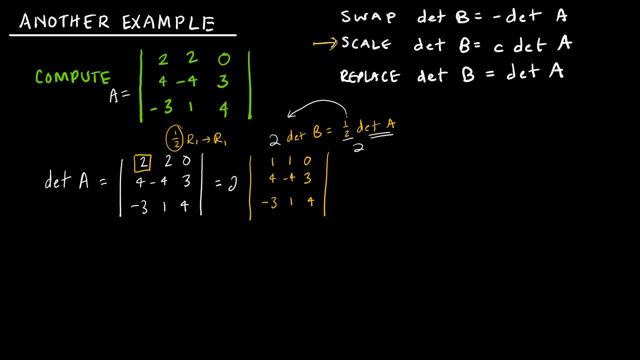 I'm saying let's take 2 times the determinant of B to be equal the determinant of A. So whatever it is that you're doing here, you're essentially doing the reciprocal multiplying by the reciprocal when you're doing it to your new matrix. So let's continue to get rid of all of that. So all I've done so far. 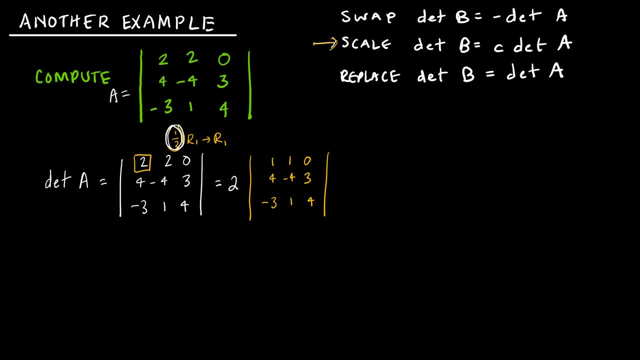 is just one row operation. Now I'm going to continue, and again, my goal here is to turn this into triangular form, which I'm not there. So I'm going to keep the 2 out front because I don't want to forget, and I can always change that too if I do another operation that tells me. 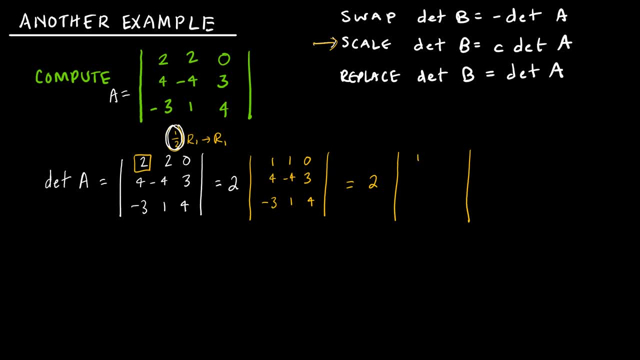 to make it negative or multiply by something else. This first row is going to remain the same. Remember, I'm trying to get zeros here in this step and so I'm going to take for row 2, I'm going to take negative 4 times row 1, which is: 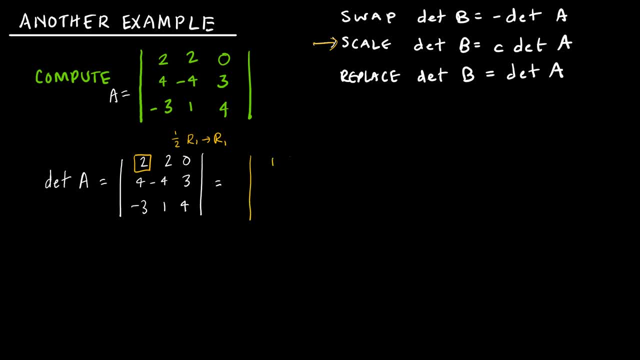 And this is the confusing part. So let me just rewrite my new matrix, so I don't screw that up. I haven't done anything else, And the question is now what? Well, I know, the determinant of this one is equal to C. 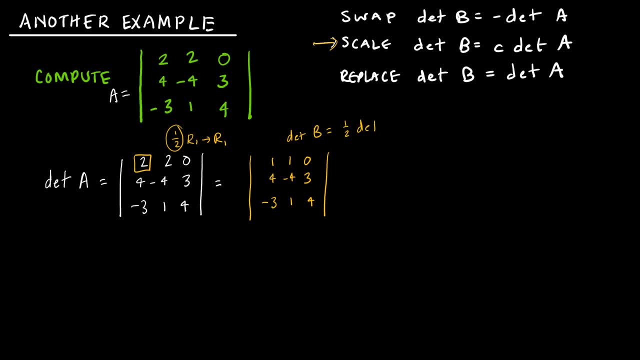 which is one half. One half the determinant of A. Here's the problem. That means a lot of people think, all right, so stick the one half here out front. but that's not the case. I'm taking half of the determinant of A. 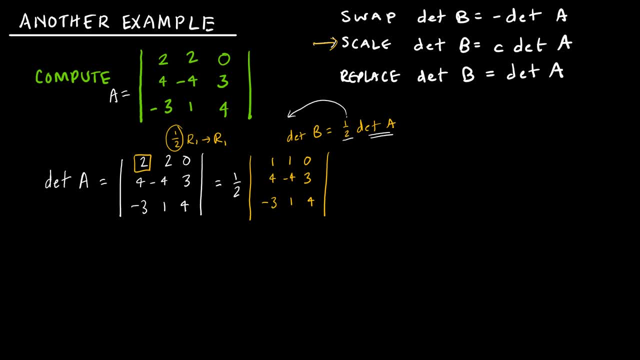 So if I needed to get the determinant of A by itself, essentially I'm saying: let's take two times the determinant of B to be equal the determinant of A. So whatever it is that you're doing here, you're essentially doing the reciprocal. 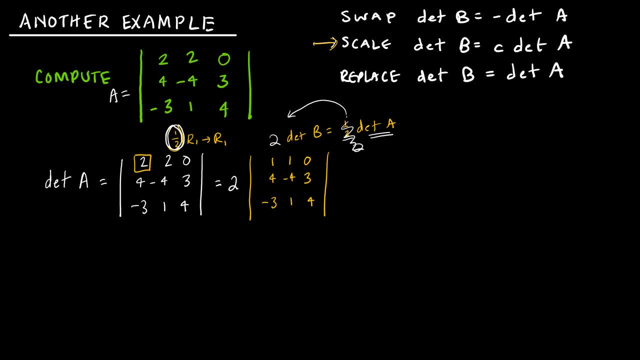 multiplying by the reciprocal when you're doing it to your new matrix. So let's continue to get rid of all of that. So all I've done so far is just one row operation. Now I'm going to continue And again, my goal here is to turn this into triangular form. 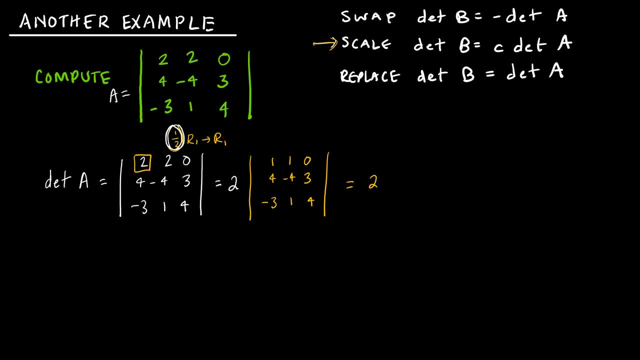 which I'm not there. So I'm going to keep the two out front because I don't want to forget, And I can always change that too if I do another operation that tells me to make it negative or multiply by something else. 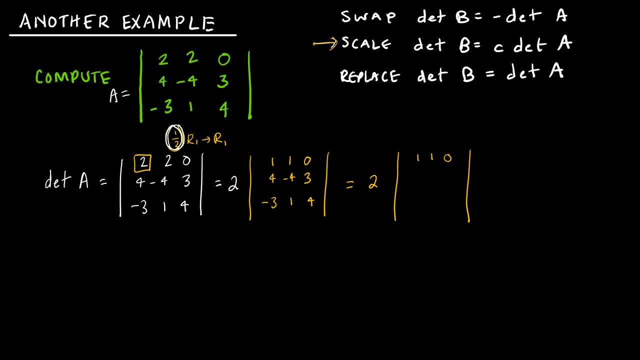 This first row is going to remain the same. Remember, I'm trying to get zeros here in this step, And so I'm going to take from row two. I'm going to take negative four times row one, which is going to give me. 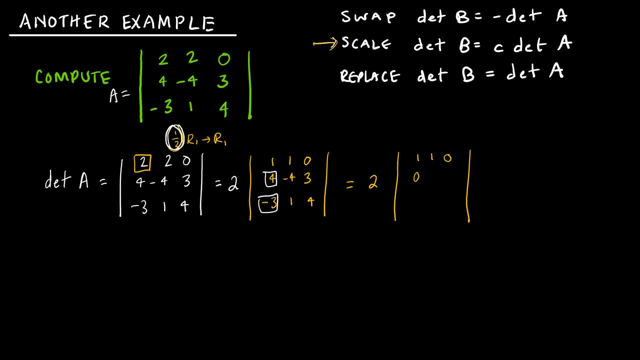 going to give me negative 4 and then plus 4 is 0.. Negative 4 plus negative 4 is negative 8, and then 0 plus 3 is 3.. And for row 3, I'm taking 3 times row 1 and adding it to row 3, so that's 3 plus negative 3, which is 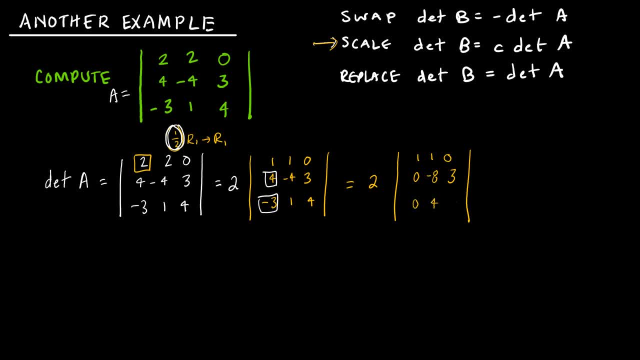 0,, 3 plus 1,, which is 4, and 0 plus 4,, which is 4.. So the two row operations that I have done in that step were both replacements and therefore I don't have to do anything else. to my determinant. 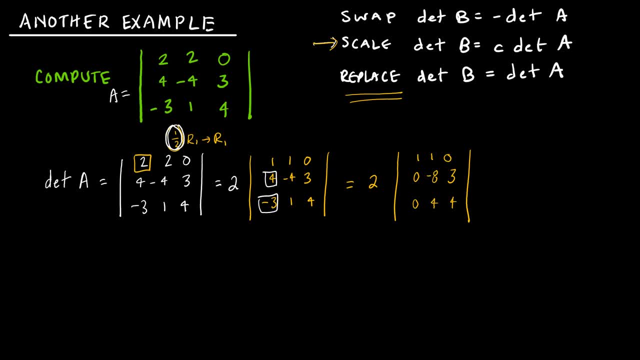 But I'm still not where I want to be. I'm trying to get to triangular form, So let's see what would happen next. I'm going to hold off on this 2 for just a second, so I'm just going to circle it so I don't forget. Let's think about what my 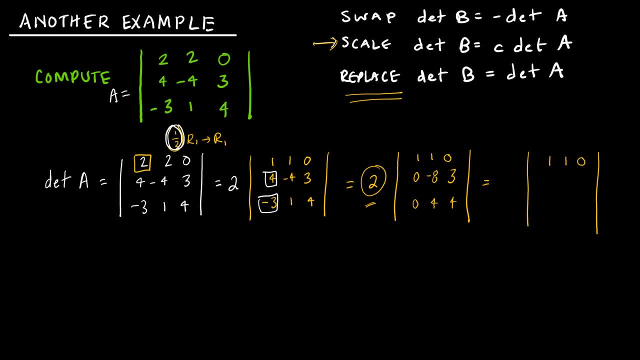 row operations would be: This first row is exactly just fine. I want the 1 first. Ideally, it doesn't have to be a 1,, it's just a matter of habit for me. So now I'm going to turn, because it's easiest. I'm going to make this guy a 0,, which means I'm going 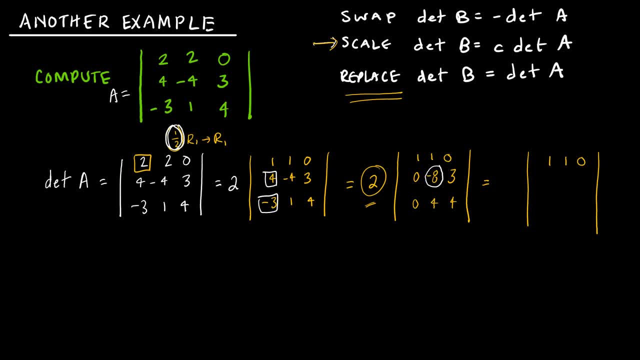 to have to end up doing another swap, but that's just fine. So I'm going to take 2 times row 2 and add it- I'm sorry- 2 times row 3 and add it to row 2, so that's 0,. 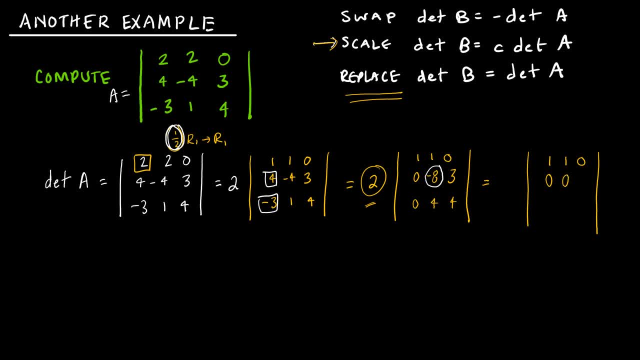 and then 2 times 4 is 8, plus 8 is 0, and then 2 times 4 is 8, plus 3 is 11.. And so keep in mind what I just did. I actually like to go back over this number one. I've already shown you how I did. 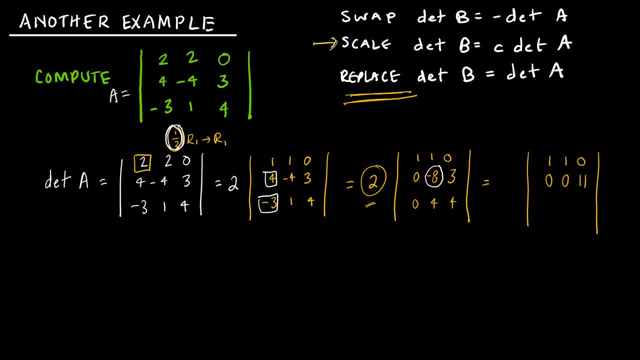 this after all of the. obviously, what I did is just a replacement and so I haven't done anything new to the determinant. But in my very last row, I'm going to take it times 1, fourth, because that's going to give me 0, 1. 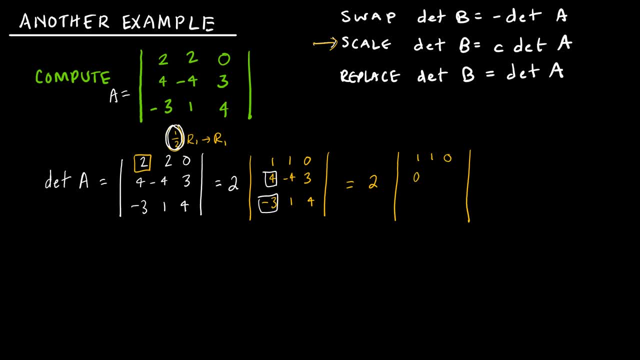 negative four, and then plus four is zero. negative four plus negative four is negative eight, and then zero plus three is three, And for row three I'm taking three times row one and adding it to row three, So that's three plus negative three. 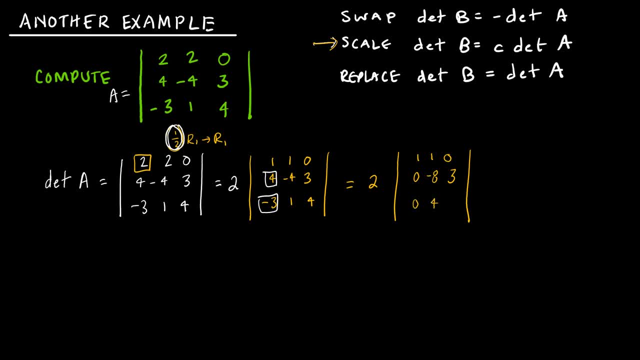 which is zero, three plus one, which is four, and zero plus four, which is four. So the two row operations that I have done in that step were both replacements and therefore I don't have to do anything else. I'm just going to go back to my determinant 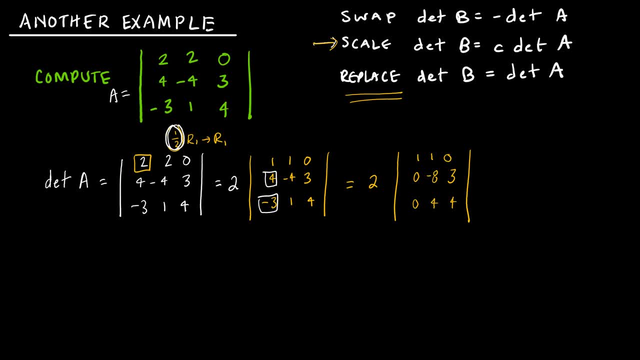 But I'm still not where I want to be. I'm trying to get to triangular form, So let's see what would happen next. I'm going to hold off on this two for just a second, So I'm just going to circle it. 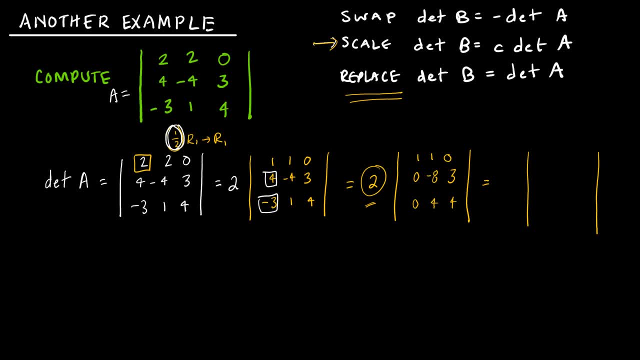 So I don't forget, Let's think about what my row operations would be. This first row is exactly just fine. I want the one first. Ideally, it doesn't have to be one, It's just a matter of habit for me. 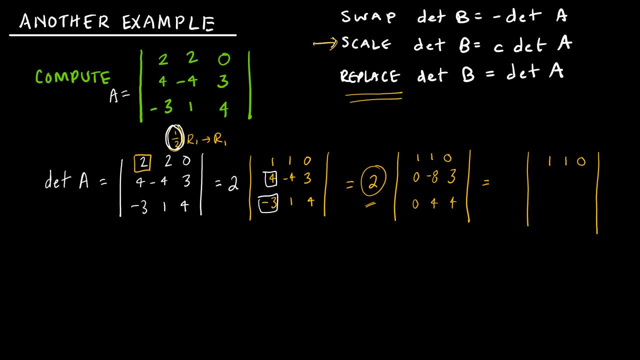 So now I'm going to- I'm going to turn because it's easiest- I'm going to make this guy a zero, which means I'm going to have to end up doing another swap, but that's just fine. So I'm going to take two times row two and add it. 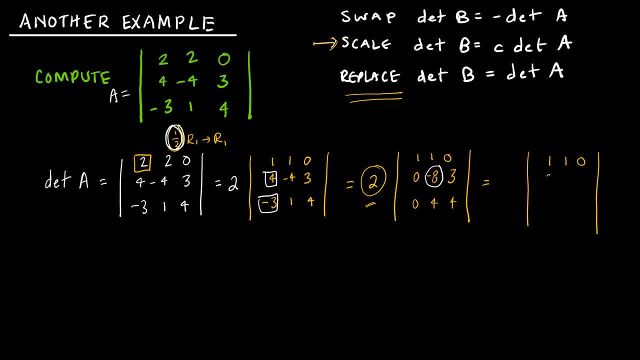 I'm sorry, two times row three and add it to row two, So that's zero. And then two times four is eight plus eight is zero, And then two times four is eight plus three is 11.. And so keep in mind. 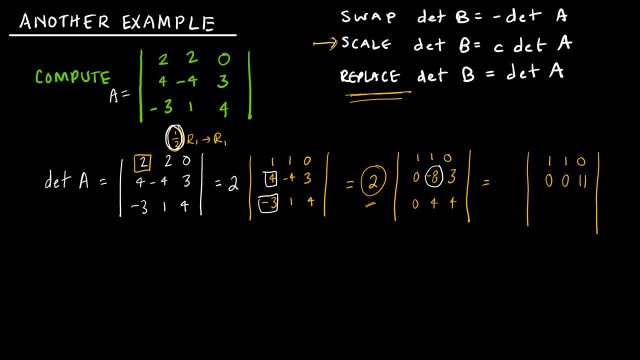 what I just did is just a replacement, And so I haven't done anything new to the determinant. But in my very last row, I'm going to take it times one, fourth, because that's going to give me zero one one. So now what's going to happen? 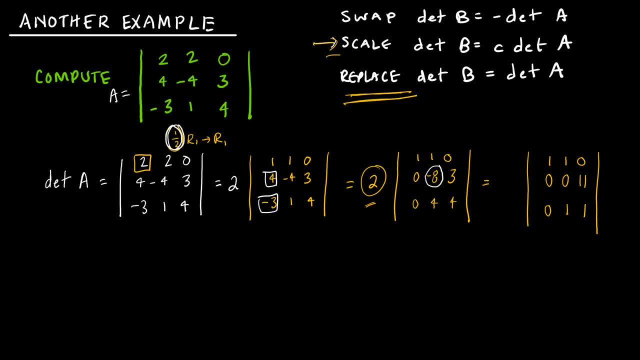 Well, that was a scale. And again, that was one fourth of row three, to be my new row three, And, just like we did before, we're taking the reciprocal of that. So now I'm multiplying by four, in addition to the two I had before. 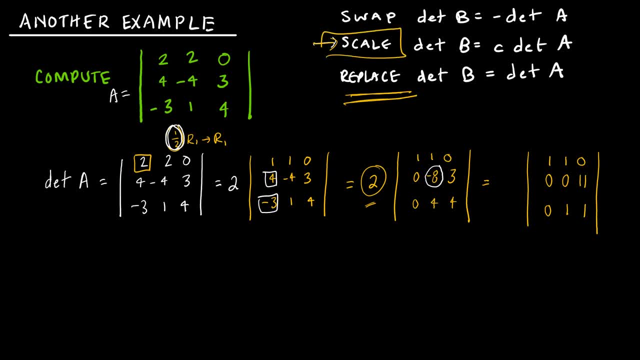 1.. So now what's going to happen? Well, that was a scale, and again that was 1, fourth of row 3, to so that it's before. we're taking the reciprocal of that. So now I'm multiplying by 4, in addition to the 2 I 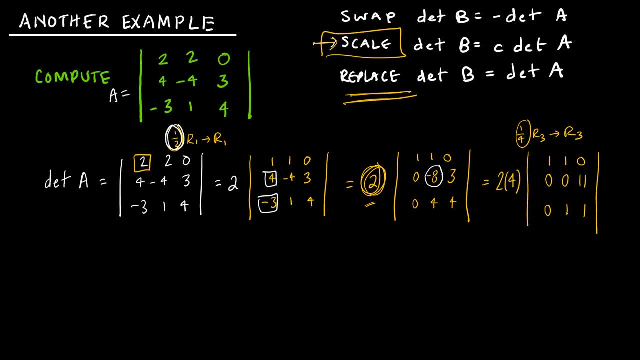 had before. So I have 2 times, 4 times- the determinant. Now I'm almost where I want to be, So I'm going to rewrite the 2.. I'm going to rewrite the 4.. And what's wrong with the matrix? 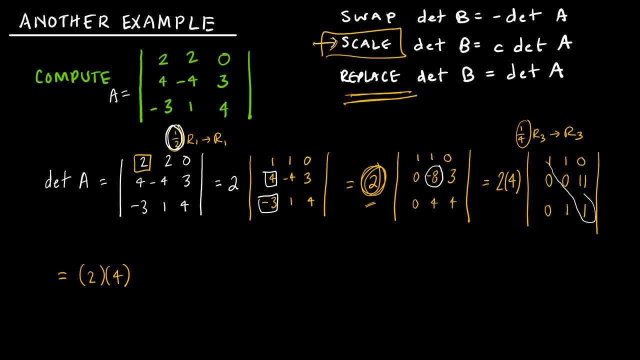 that I have. Well, it's not quite triangular form yet, but all I'm going to need to do is do a swap, an interchange. So this guy is going to stay the same. I'm going to swap or interchange rows 2 and 3.. So that's 0, 1, 1, 0, 0, 11.. What happens when I do a swap? I'm going to take 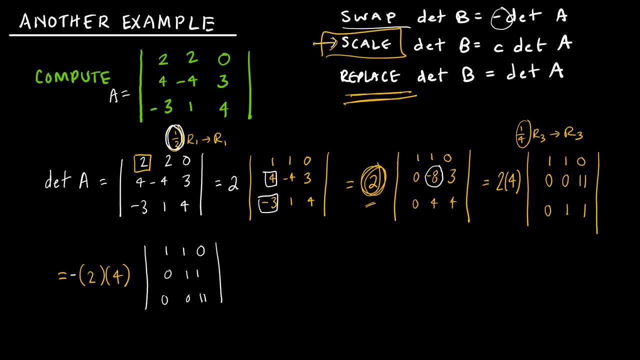 negative. So now I have triangular form which tells me my determinant is negative Negative 2 times 4.. And then my diagonal is 1 times 1 times 11.. So if I multiply negative 2 times 4 times 1 times 1 times 11, I get negative 88. And that is in fact my determinant. 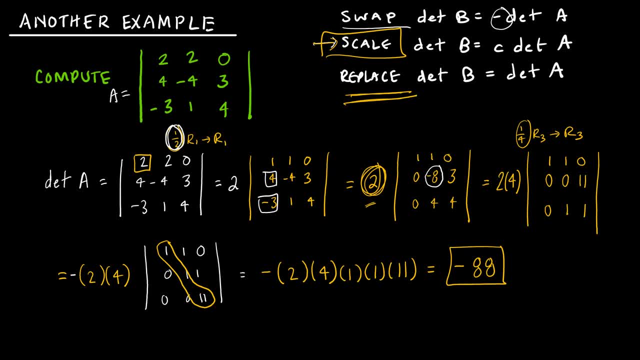 This is how I would like you to show your work. I want to see that you are putting these values out front, So don't turn this into 8 yet. I'm going to show you how to do that, So I'm going to. 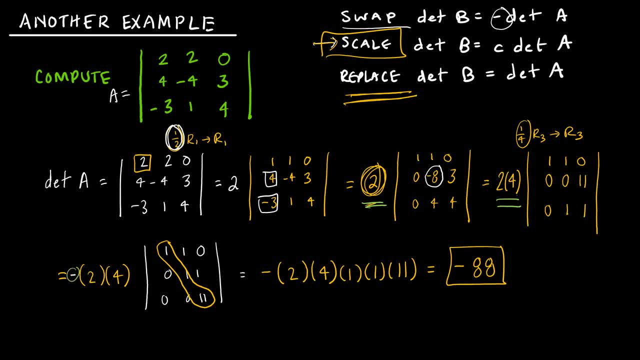 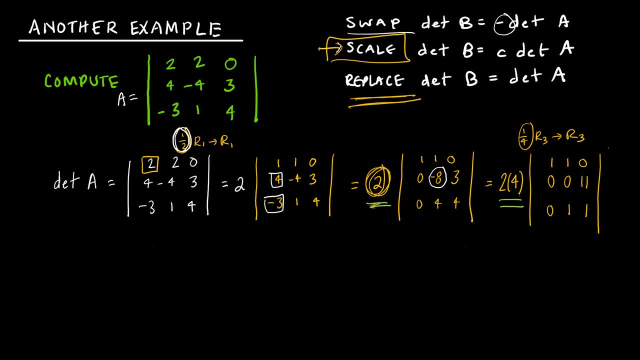 go ahead and keep it as 2 times. 4. Keep the negative out front. I want to see this as your work as you continue through your examples. I wanted to look at the same example, real quick, one more time, because we got it to this: 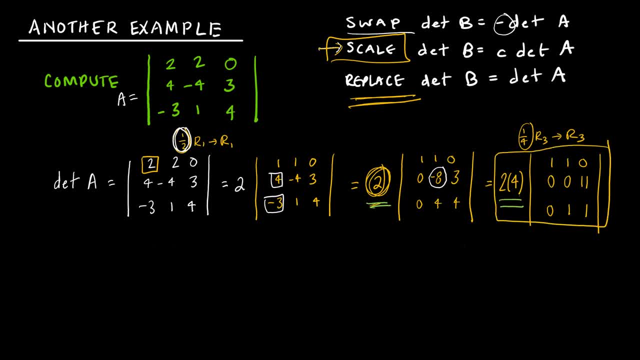 point, And then my next step was to do a swap or an interchange to turn it into a triangular form. I did want to point out to you that you don't always have to put it in triangular form. So, for instance, I'm going to keep my 2 times 4, and what if I then did cofactor expansion? 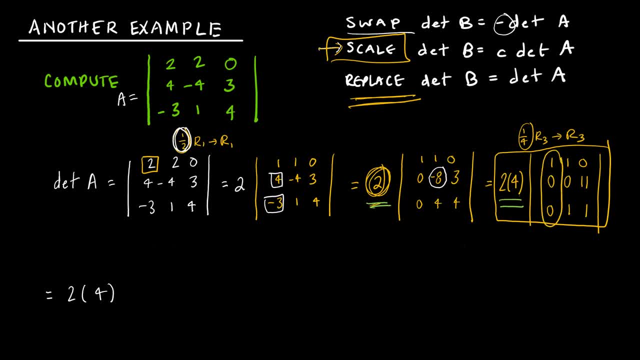 for this column. Well, that would tell me that I'm going to take negative 1 to the 1 plus 1, and then I'm taking the determinant of zero, 11, 1, 1, and then the other values are zeros. 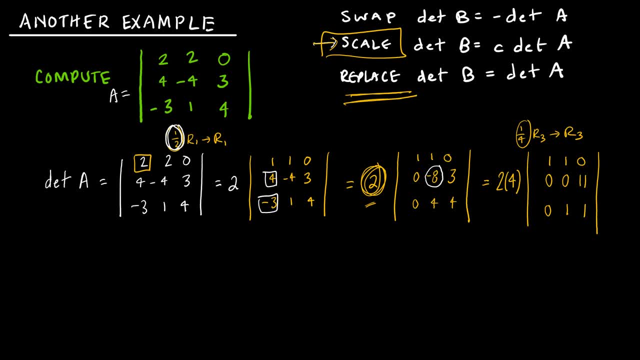 So I have two times, four times, the determinant. Now I'm almost where I want to be, So I'm going to rewrite the two, I'm going to rewrite the four. And what's wrong with the matrix that I have? Well, it's not quite triangular form yet. 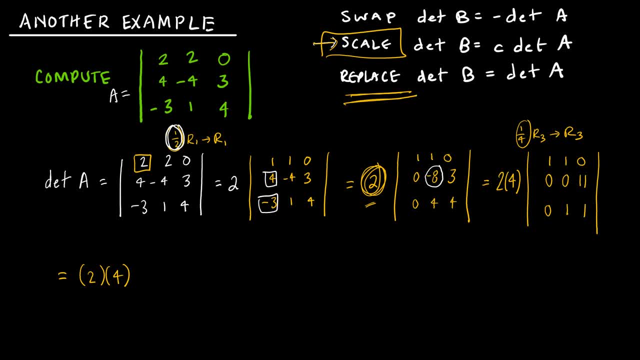 but all I'm going to need to do is do a swap and interchange, So this guy is going to stay the same. I'm going to swap or interchange rows two and three, So that zero one one, zero zero eleven. What happens when I do a swap? 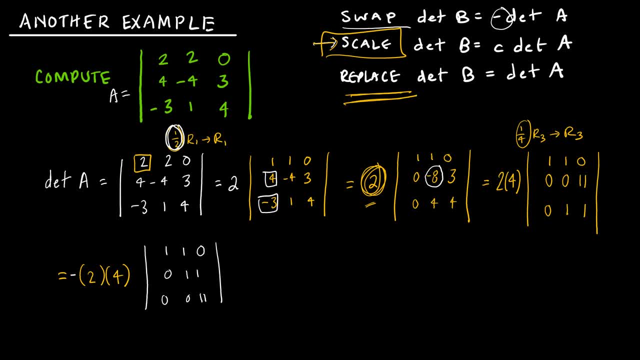 I'm going to take negative. So now I have triangular form Which tells me my determinant is negative two times four And then my diagonal is one times one times 11.. So if I multiply negative two times four times one times one times 11,, 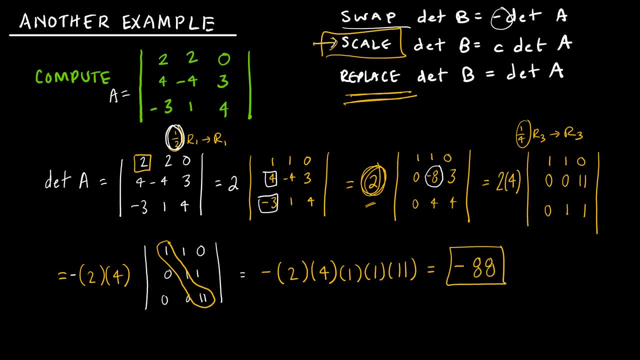 I get negative 88, and that is, in fact, my determinant. This is how I would like you to show your work. I want to see That you are putting these values out front, So don't turn this into eight yet. Go ahead and keep it as two times four. 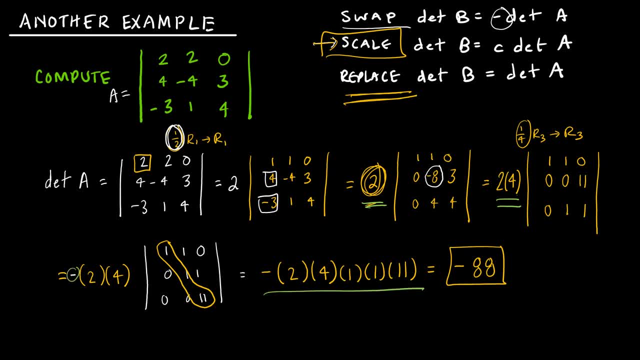 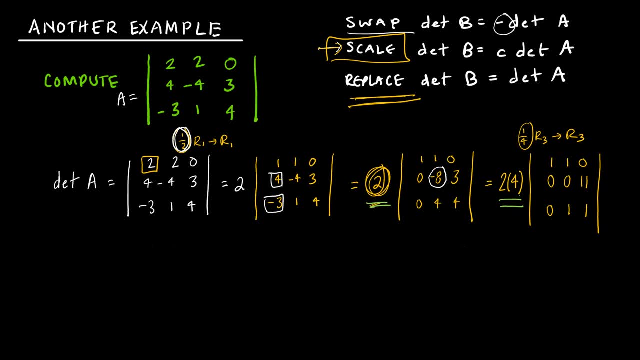 Keep the negative out front. I want to see this as your work, as you continue through your examples. I wanted to look at the same example, real quick, one more time, because we got it to this point, And then my next step was to do a swap or an interchange. 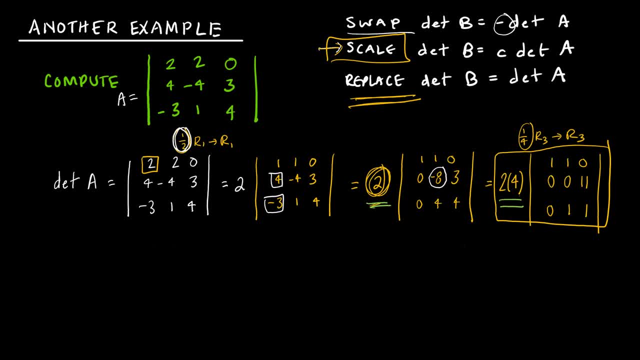 To turn it into a triangular form. I did just want to point out to you that you don't always have to put it in triangular form. So, for instance, I'm going to keep my two times four. And what if I then did cofactor expansion for this column? 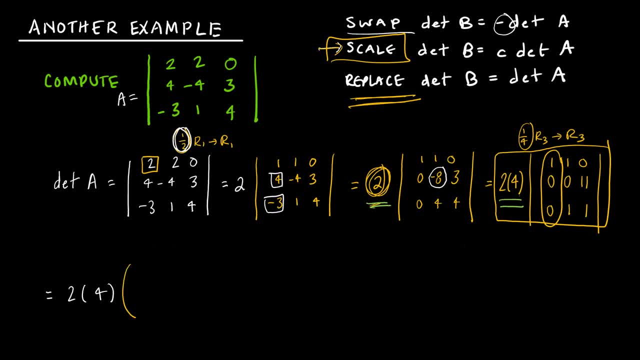 Well, that would tell me that I'm going to take negative one to the one plus one, And then I'm taking the determinant of zero, eleven one one, and then the other values are zeros. So it'd be plus zero, plus zero, which I don't need to do. 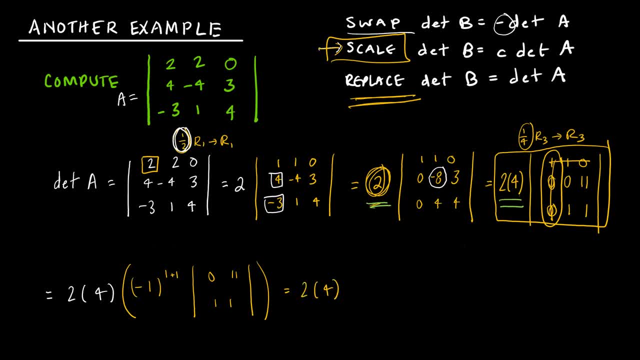 So now I could have two times four. negative one to the second would be: I'm just going to go ahead and write negative one to the second and then zero times one. So that gives me two times four times negative one squared, which is one. and then what's happening here? 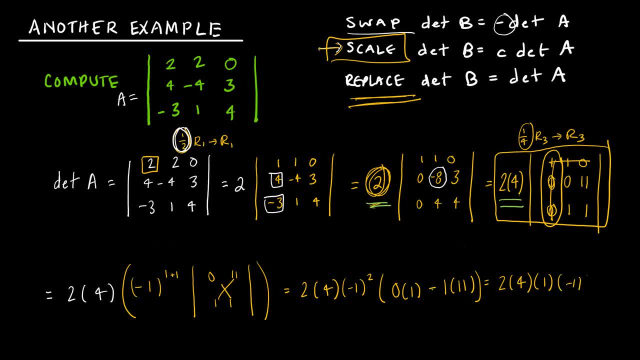 I have zero minus eleven, which is negative eleven, And if I take two times four times one times negative eleven, I get negative eighty eight, which is the exact same solution I had before. Here's one for you to try. You can choose to use cofactor expansion. 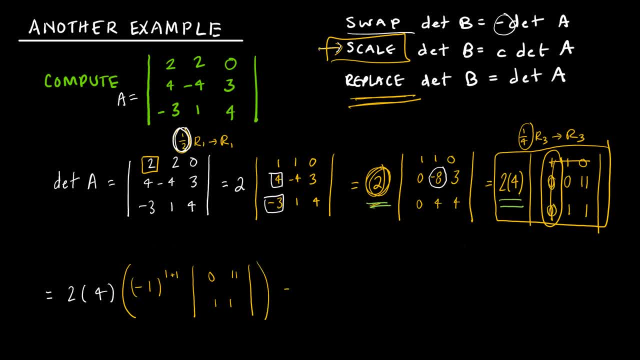 so it would be plus 0 plus 0,, which I don't need to do. So now I could have 2 times 4, negative 1 to the second would be. I'm just going to go ahead and write negative 1 to the second. 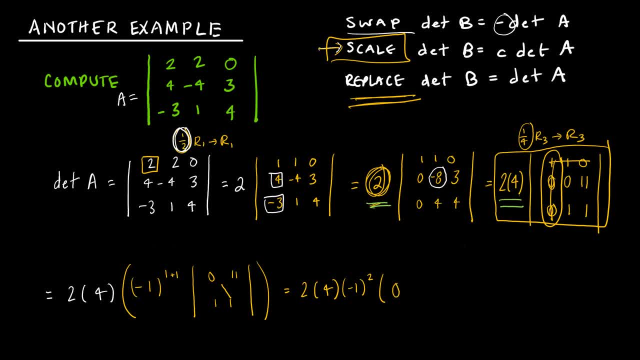 and then zero times 4.. 1 minus 1 times 11, so that gives me 2 times 4 times negative 1, squared, which is 1. and then what's happening here? I have 0 minus 11, which is negative 11, and 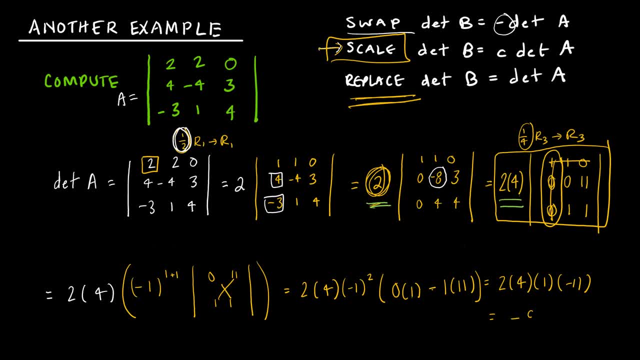 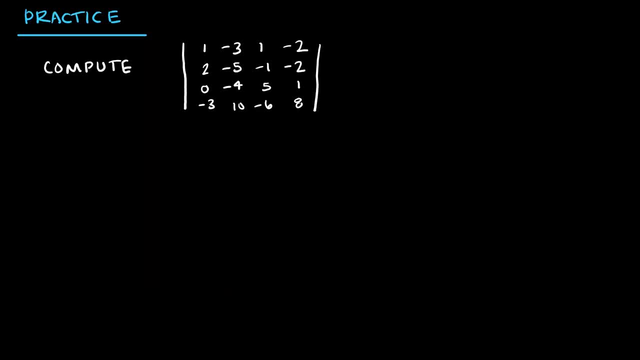 if I take 2 times, 4 times, 1 times, negative 11, I get negative 88, which is the exact same solution I had before. here's one for you to try. you can choose to use cofactor expansion, you can use row operations, you can use a mixture of. 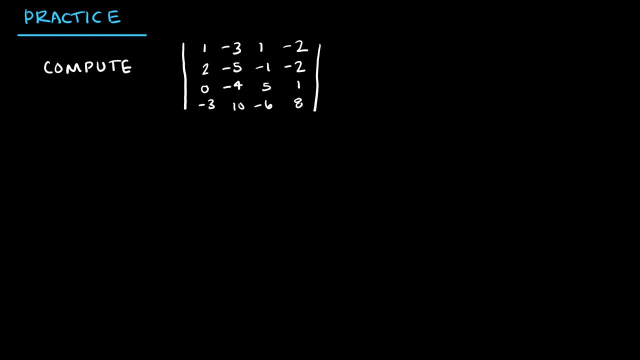 both of them. do whatever works for you in this question. when you're ready and have tried the question, press play to see how you did so. first thing I would do is say that I'm finding the determinant of a and I'm going to do some row operations right off the bat, so I'm going to keep my first row. 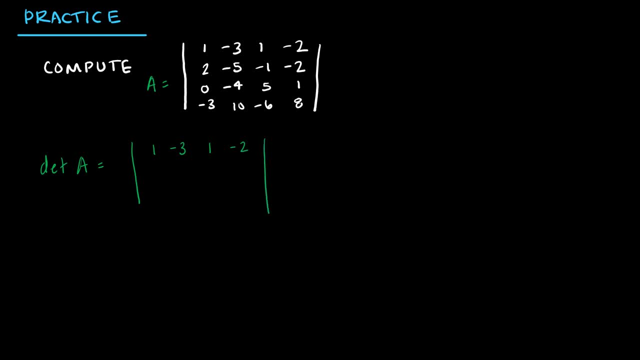 exactly as it is. I'm going to add negative two of my first row to my second row to get zero one negative three and two. this guy is already how I want it and I'm going to take three times my first row. so three times one plus three, that's negative nine plus. 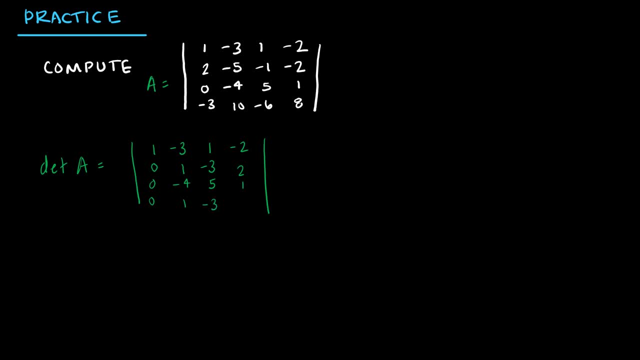 three times one plus four, that's negative. nine plus three, that's negative plus 10,, that's 3 plus negative 6, and that's negative 6 plus 8.. From here, have I done anything in that last example or the last steps that changed my? 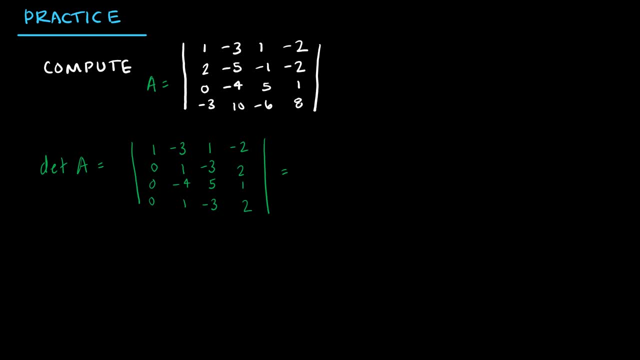 determinant. Well, I did two replacements and we know replacements don't change it, so nothing has happened. So now I might choose. since I'm not restricted by a specific way to do this, I might choose to do some cofactor expansion using that first column, because that's a lot of 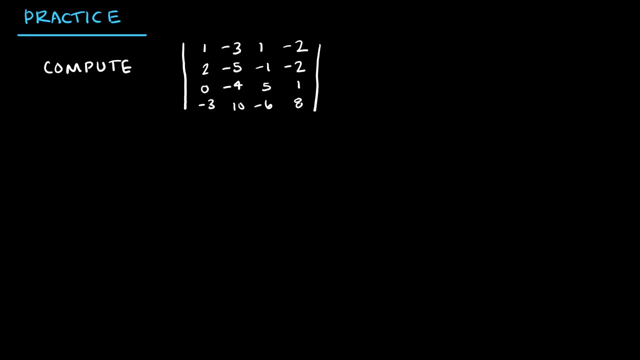 You can use row operations. You can use a mixture of both of them. Do whatever works for you in this question. When you're ready and have tried the question, press play to see how you did So. first thing I would do is say that I'm finding the determinant of a 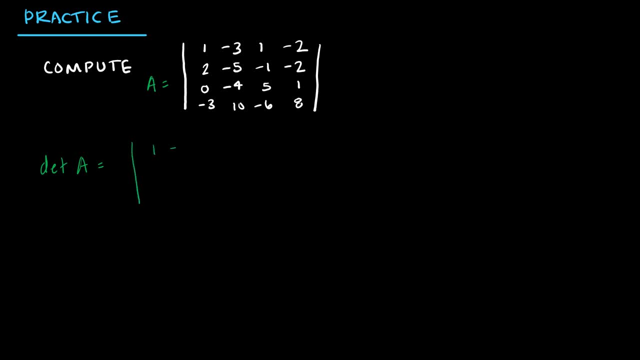 and I'm going to do some row operations right off the bat, So I'm going to keep my first row exactly as it is. I'm going to add negative two of my first row to my second row to get zero one negative three and two. 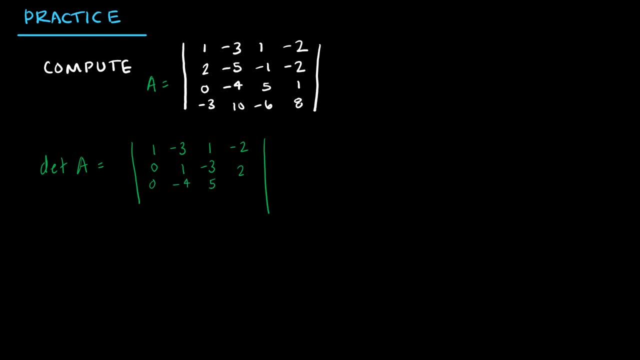 This guy is already how I want it And I'm going to take three times my first row. So three times one plus three, that's negative nine plus ten, That's three plus negative six and that's negative six plus eight From here. 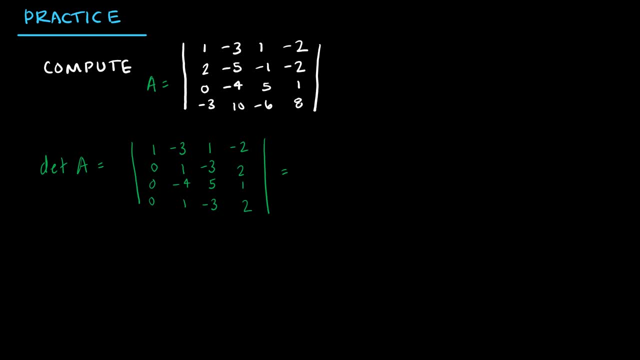 Have I done anything in that last example or the last steps that changed my determinant? Well, I did two replacements, and we know replacements don't change it, So nothing has happened. So now I might choose- since I'm not restricted by a specific way to do this. 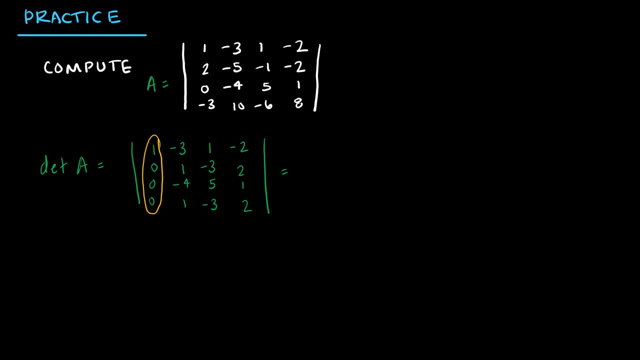 I might choose to do some cofactor expansion using that first column, because that's a lot of zeros. So that would tell me that I'm taking one Times negative, one to the One plus one, And then the determinant of One negative three, two negative four five. one one negative three, two. 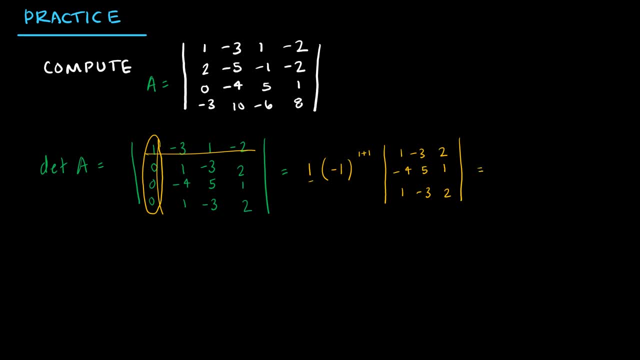 So what do I have so far? I have one and I have negative one squared, which is one. So really all I'm doing is Finding the determinant of this new matrix, And that's a little bit more manageable. but let's maybe do some row operations. 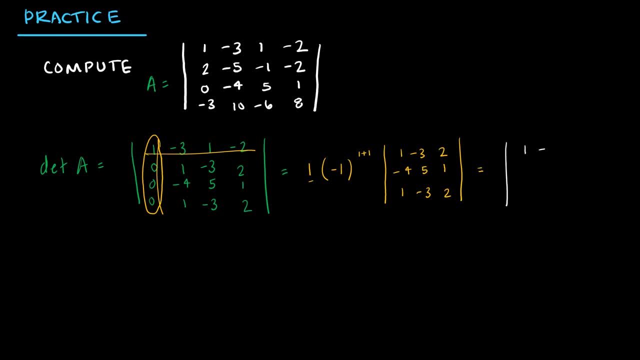 So I'm going to take The first row and keep it exactly the same. The second row, I'm going to take four times the first row and add it to the second row, So that gives me zero negative twelve plus five And eight plus one. 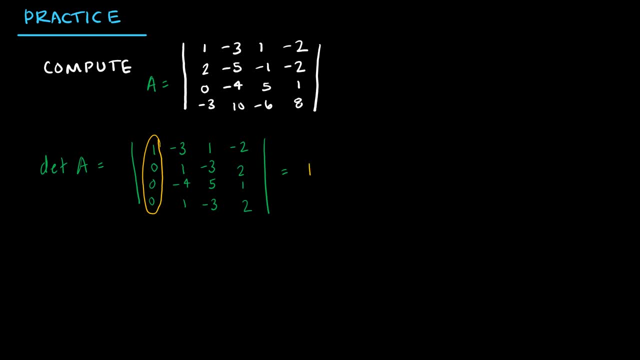 zeros. So that would tell me that I'm taking 1 times negative 1 to the 1 plus 1, and then the determinant of 1, negative 3, 2, negative 4, 5, 1, 1, negative 3, 2.. 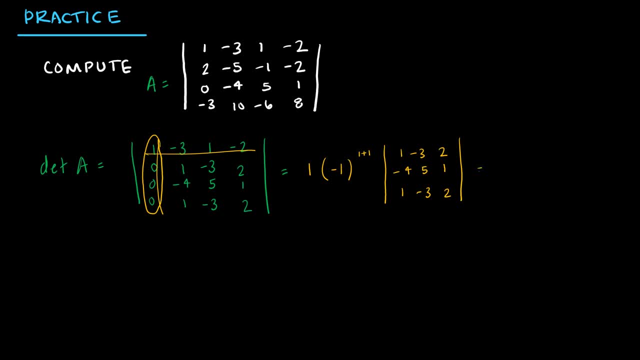 So what do I have so far? I have 1, and I have negative 1 squared, which is 1.. So really, all I'm doing is finding the determinant of this new matrix, and that's a little bit more manageable. but let's maybe do some row operations. So I'm going to take the first row and keep it exactly. 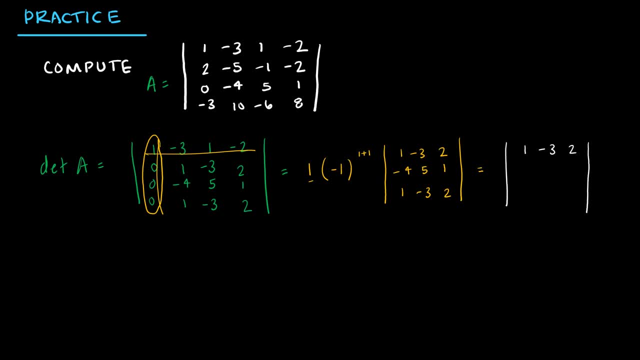 the same, The second row. I'm going to take 4 times the first row and add it to the second row, So that gives me 0, negative 12 plus 5, and 8 plus 1.. And then I'm going to take row 1 minus row 3,. 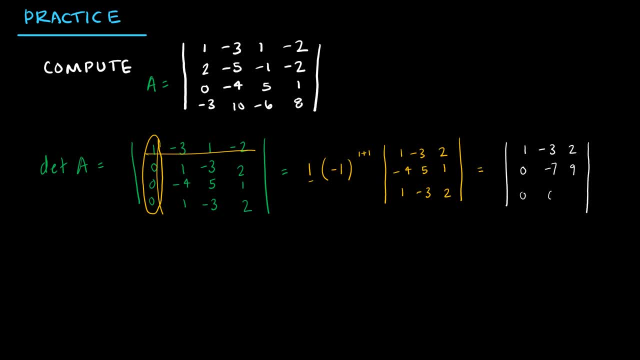 which gives me 0, 0, 0.. So now what? Well, hopefully it's very clear to you, but if not, let's just go with it. Let's say, I want to do a cofactor expansion with this row. Well, that's going to give me 0 times. who cares? 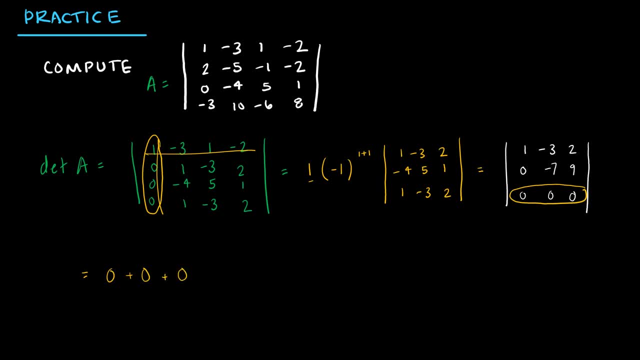 plus 0 times again, who cares? plus 0 times who cares, which means my determinant is in fact 0. And I did that in not too many steps. So this one, which I actually did two steps in one on that. 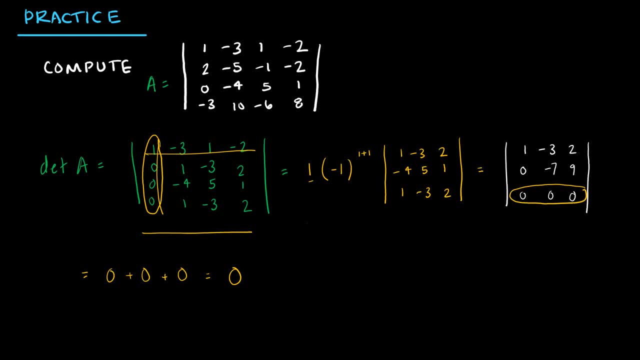 but that's okay, Don't do three steps, do two steps And then another step, that second step, that's the third step, And then I found my solution in sort of the fourth step. So I found that my solution is, in fact, 0.. Here are two more properties that I want to go through. 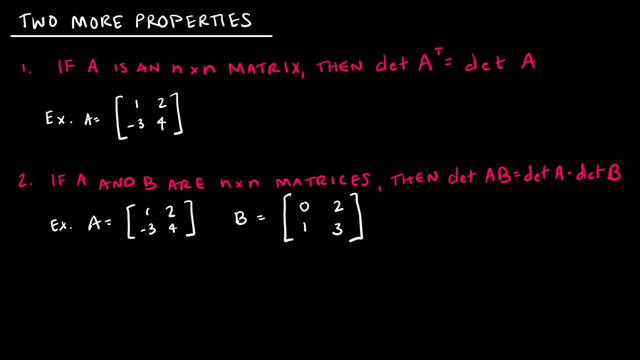 with you. And again, these do require proof, and those proofs are in your text. I'm not going to spend time on those proofs with you. I just want to go over the properties and verify with you that they do in fact hold. So, for instance, the first one says: if A is an n by n matrix. 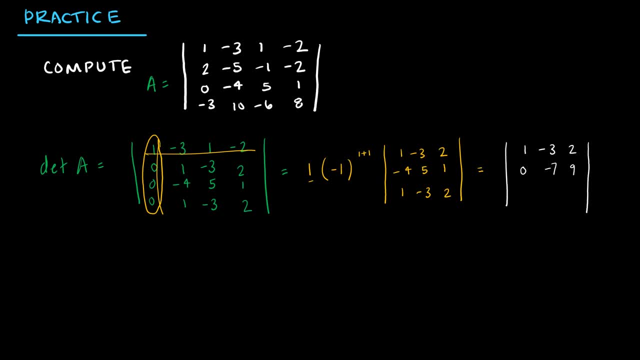 And then I'm going to Take row one minus row three, Which gives me zero, Zero, Zero. So Now what? Well, hopefully it's very clear to you, But if not, let's just go with it. Let's say: I want to do a cofactor expansion with this row. 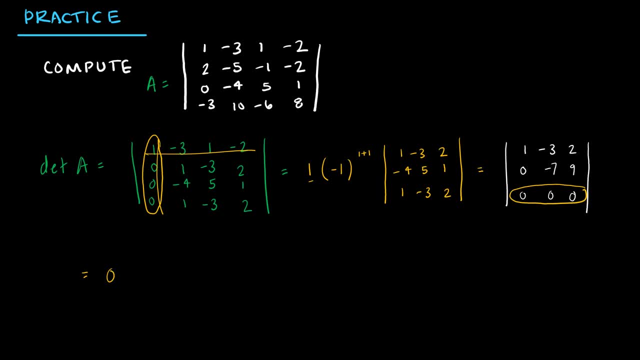 Well, that's going to give me zero times. Who cares? plus zero times again, Who cares? plus zero times. Who cares? Which means my determinant is in fact zero, and I did that in not too many steps, So this one, which I actually did two steps in one on that, but that's okay. 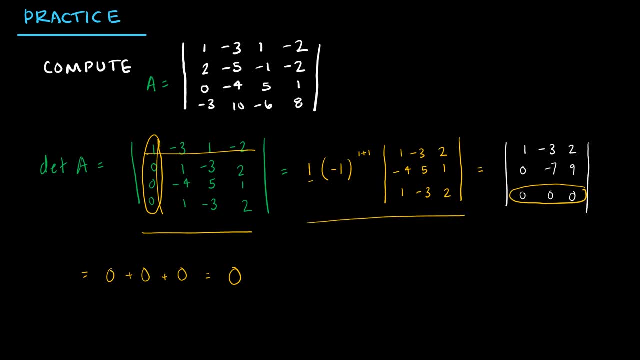 Don't do three steps, do two steps and then another step, that second step, That's the third step, And then I found my solution, in sort of the fourth step. So I found that my solution is, in fact, zero. Here are two more properties that I want to go through with you. 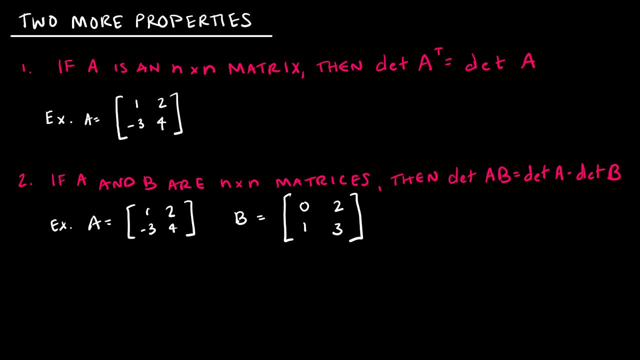 And again, these do require proof, and those proofs are in your text. I'm not going to spend time on those proofs with you. I just want to go over the properties and verify with you that they do in fact hold. So, for instance, the first one says: if a is an end by end Matrix, then the determinant of a transpose is equal to the determinant of a. 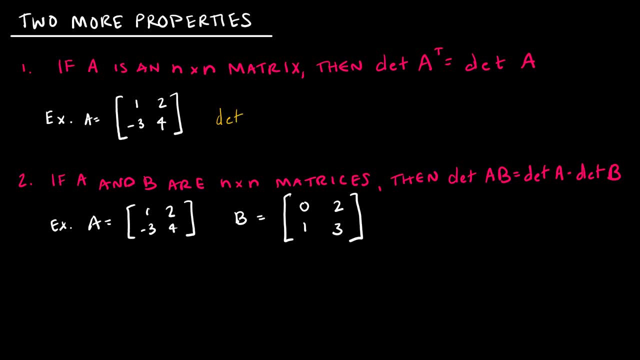 So to find the determinant of a, I'm just going to use our Very simple formula that says: one times four is four minus negative. three times two is negative six and that gives me ten. So what is a transpose? Remember, a transpose takes rows and turns them into columns, and columns and turns them into rows. 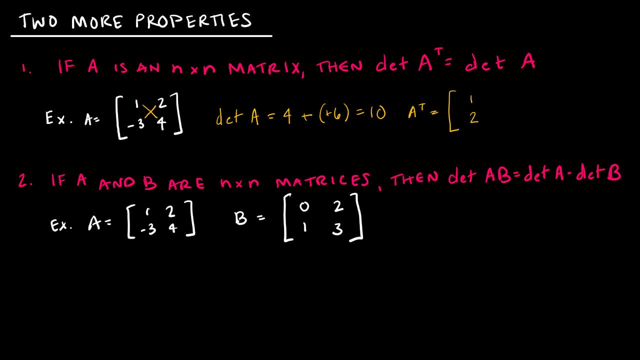 So one, two as a row becomes one, two as a column- negative three. four as a row becomes negative three, four as a column. And now I'm going to find the determinant Of a transpose which is one times four or four minus two times negative three, which is negative six. 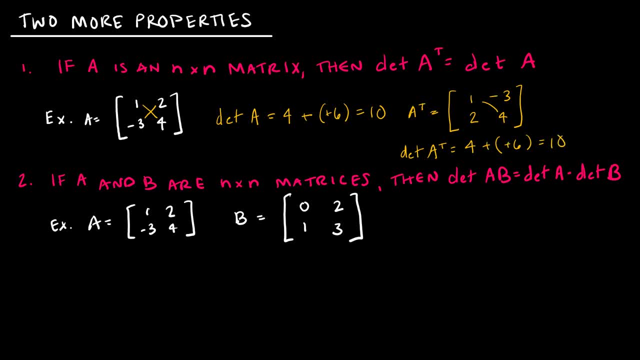 And I do in fact get ten, And it's very clear to see why I'm taking the exact same values. So again, this is not a proof. The proof is in your textbook, but this is just showing you that in fact, it does hold true. 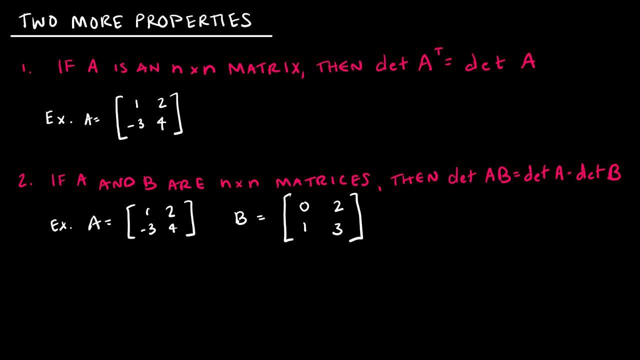 then the determinant of A transpose, it's equal to the determinant of A. So to find the determinant of A, I'm just going to use our very simple formula that says: 1 times 4 is 4, minus negative. 3 times 2 is negative 6, and that gives me 10.. 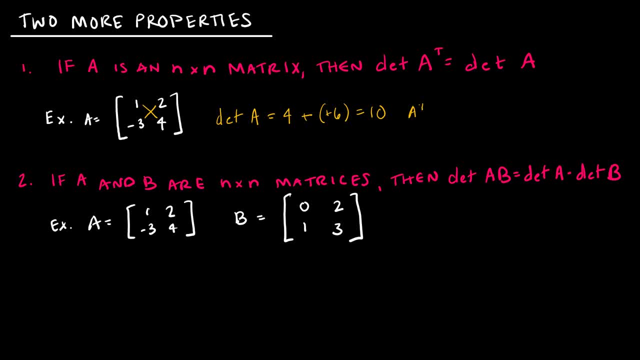 So what is A transpose? Remember: A transpose takes rows and turns them into columns, and columns and turns them into rows. So 1, 2 as a row becomes 1, 2 as a column. Negative. 3, 4 as a row becomes negative 3, 4 as a column. 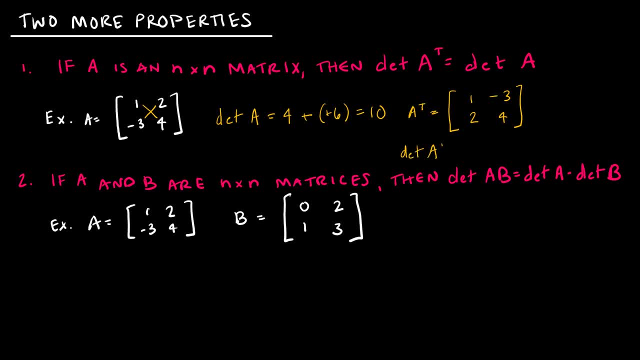 And now I'm going to find the determinant of A transpose which is 1 times 4, or 4, minus 2 times negative 3,, which is negative 6. And I do in fact get 10.. And it's very clear to see why I'm taking the exact same values. 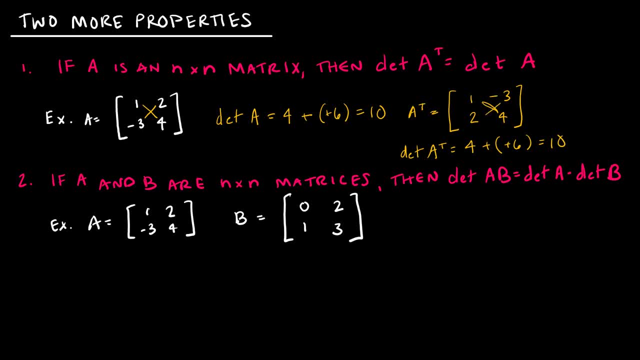 So again, this is not a proof. The proof is in your textbook, but this is just showing you that in fact, it does hold true. So now let's take a look at our last property for this section, which is, if A and B are n by n matrices. 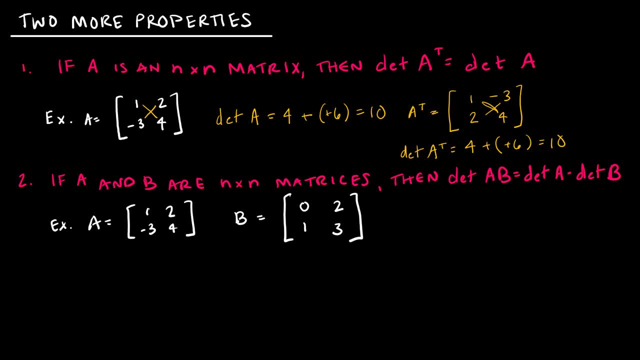 then the determinant of the product of A and B is equal to the product of the determinants. So we already know that the determinant of A is equal to 10, as we found it above, and it's the same matrix. The determinant of B can be found easily by taking 0, minus 2, or negative 2,. 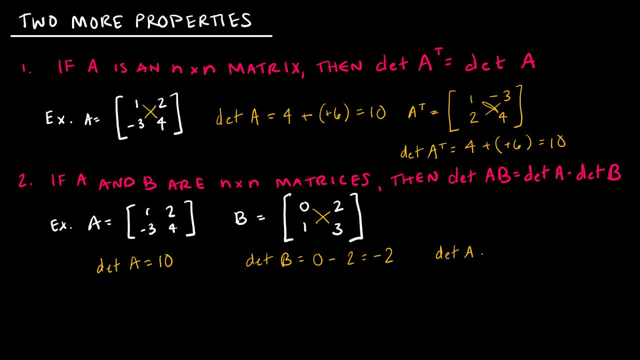 which means determinant of A times determinant of B is equal to 10 times negative 2 or negative 20.. So now I need to do a little bit of math, because I need to find what is AB, and then I'm going to find the determinant of that product. 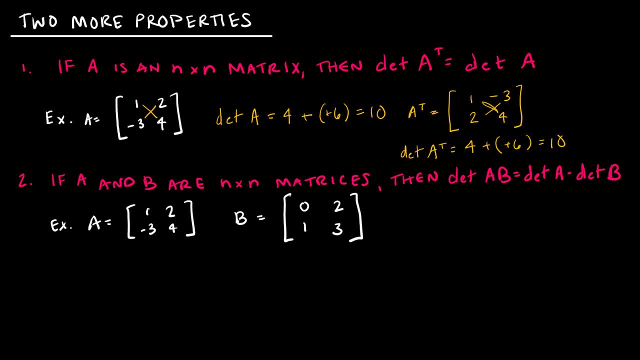 So now let's take a look at our last property For this section, which is, if a and b are end by end matrices, Then the determinant of the product of a and b is equal to the product of the determinants. So we already know that determinant of a is equal to 10, as we found it above, and it's the same matrix. 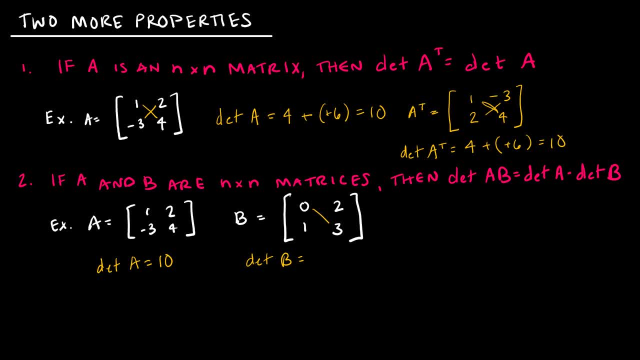 The determinant of b can be found easily by taking zero minus two or negative two, which means determinant of times. determinant of B is equal to 10 times negative 2 or negative 20.. So now I need to do a little bit of math, because I need to find what is AB, and then I'm 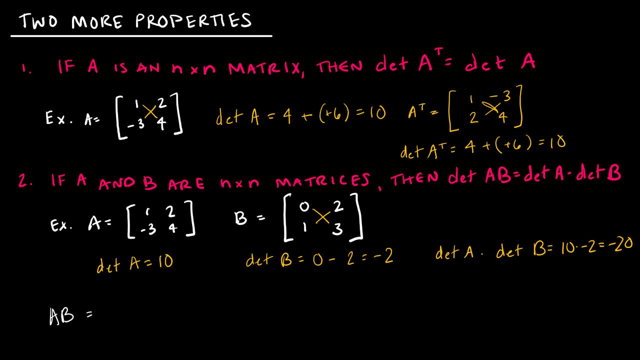 going to define, find the determinant of that product. So A times B is. I'm going to take this row: times the first column, so that would be 1 times 0 or 0, plus 2 times 1, which is 2, and then times the next column, which is 1 times 2 or 2 plus. 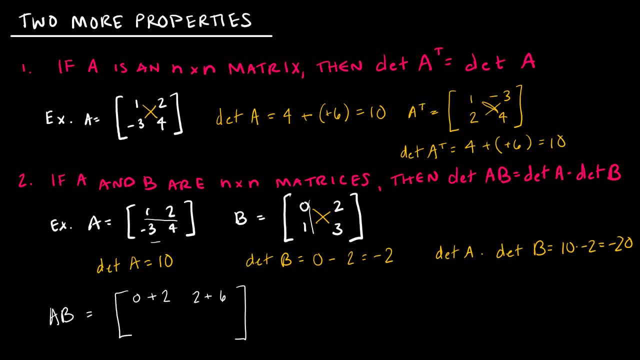 2 times 3, which is 6.. Now I'm moving on to my next row. negative 3 times 0 is 0 plus 4 times 1 is 4, and second row, second column, would be negative 3 times 2, or negative 6 plus 4 times 3, which is 12.. That gives me my new product matrix. 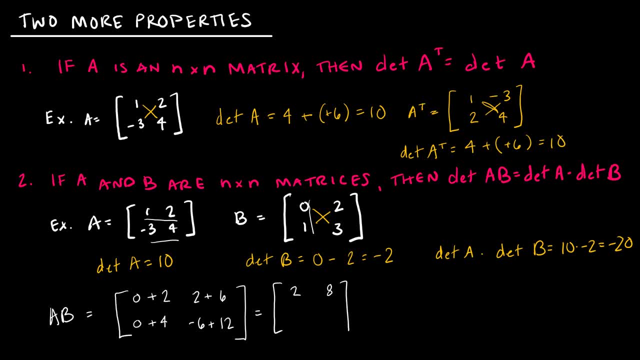 of B, So I have 2,, 8,, 4,, 6.. Now I want to find the determinant of AB, and that would be 2 times 6 minus 4 times 8, which would be 12 minus 32, which would be negative 20.. 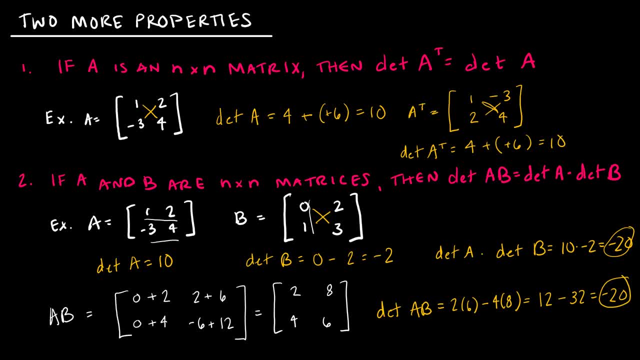 So again, I'm just showing you the properties of AB and then I'm just showing you that those properties do hold true. Those proofs are in your textbook, so feel free to take a look. 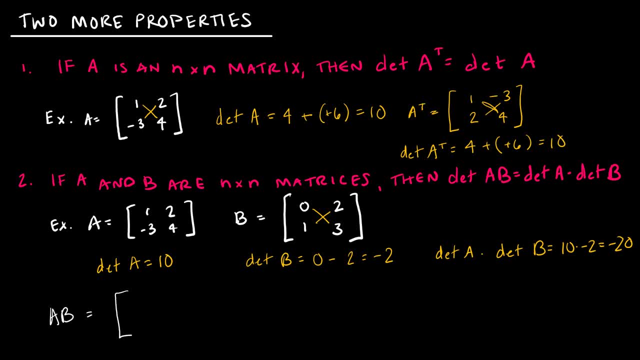 So A times A, A times B is. I'm going to take this row times the first column, so that would be 1 times 0 or 0, plus 2 times 1,, which is 2, and then times the next column, which is 1 times 2 or 2, plus 2 times 3,, which is 6..